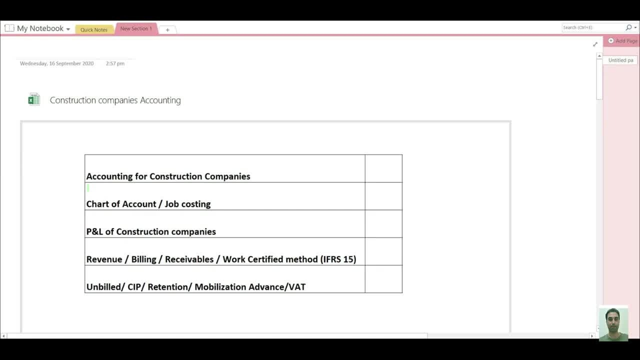 Hi, this is Ishwar Khan, and in today's session I'm going to discuss with you accounting for construction companies. So it will be a kind of advanced level- not that much advanced level, but you must have accounting background or experience working as an accountant, or you must have experience in this field to understand this session. So it will, this session will definitely help you out. So what we are going to discuss in this session is: I will discuss with you chart of account for a construction company. 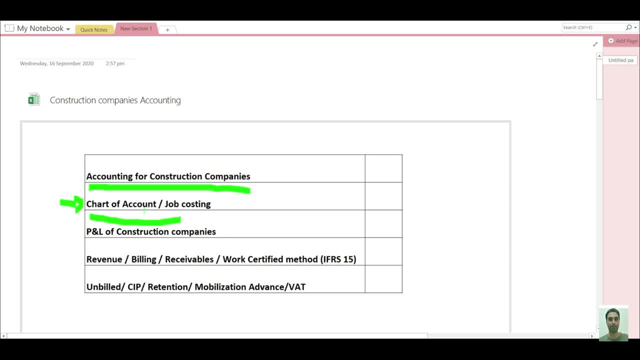 How does it look like Then, even if you are using Tally, QuickBook or any ERP system? So how you will design your chart of account, I will look, have a brief look at that as well. After that we will discuss the job costing concept, Not in that much detail, but we will look through it. How does it works Then? I will going to show you the P&L of construction company. How does it look like? And then at the end, 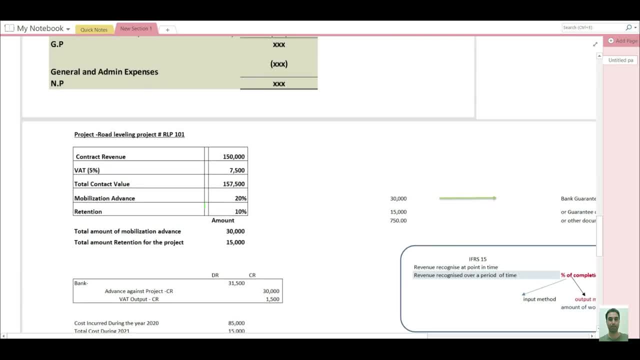 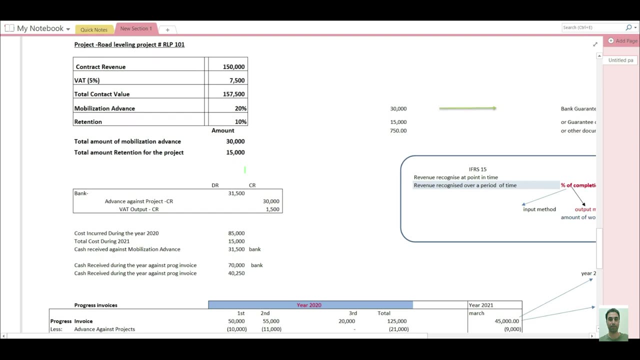 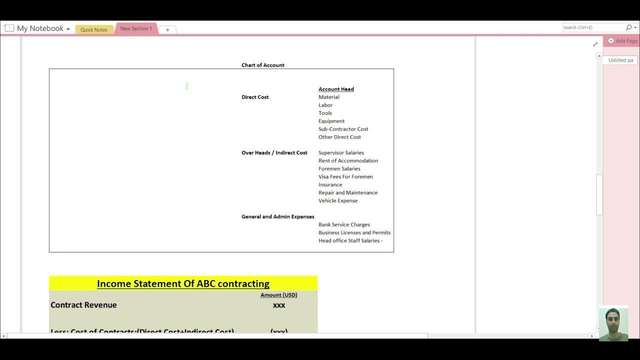 I'm going to show you, with the help of an example, How will you record all these transactions if you have a contract, and how you will implement that contract. that has retention, vet, mobilization, advance and all these things, with even their effect, journal entries and all this stuff I will. So this is a chart of account for construction company. Okay, before going to chart of account, let's do these two things together: Chart of account and income statement of a construction company. 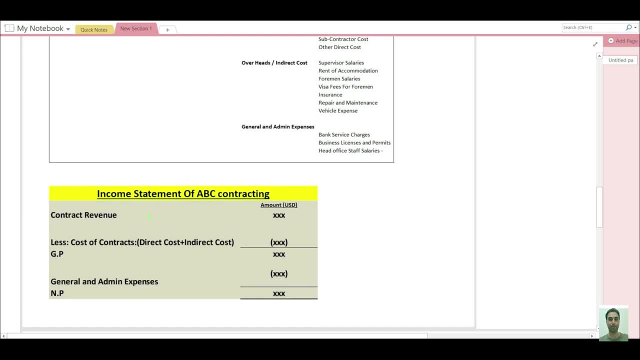 How far as contracting industry income statement is concerned, you can look at that, But how does it appears It has contract revenue? contract revenue is revenue from your project. Okay, you have a project. the revenue of that project you will record here. Then you deduct from that to your cost of contracts or cost of your projects. These are all the costs that are incurred specifically to that project. But this project has to be recorded. 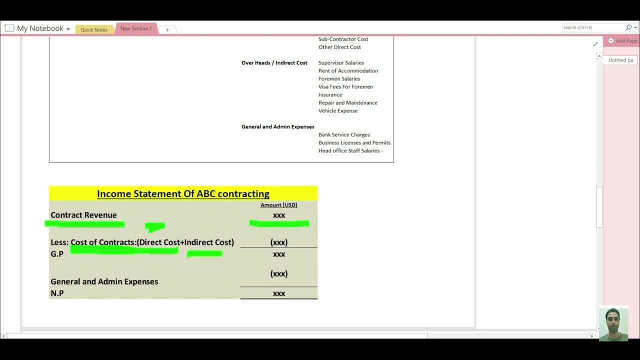 parts. one is direct cost here, the other is indirect cost. okay, so this direct cost and indirect cost both form the cost of the contract. so i want to explain to you a little bit more what is direct cost and what is indirect cost. but keep in mind these two cost are cost of goods sold. 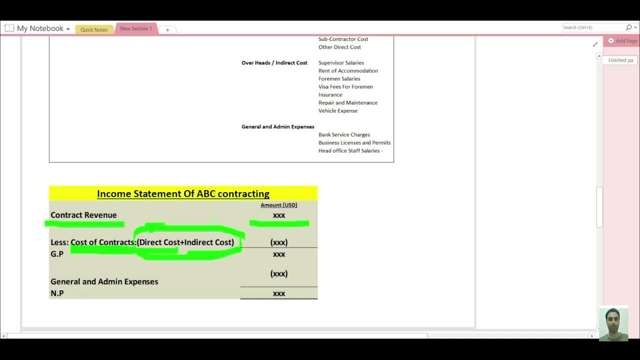 are directly associated with the project. now you will be wondering if these both cost direct cost and indirect cost. we also call this direct, indirect cost as overheads. okay, and these direct cost are not overheads. they are directly associated to, that can be directly allocated to the projects. 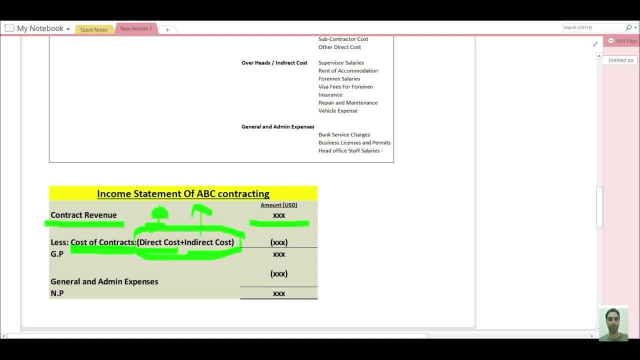 now let's see. what does it mean what i am trying to say over here- direct cost and indirect cost. okay, this indirect cost or direct indirect cost or overhead. let me start with the direct cost. direct cost is the cost that are directly allocated to that specific project, like here in the chart of account you. 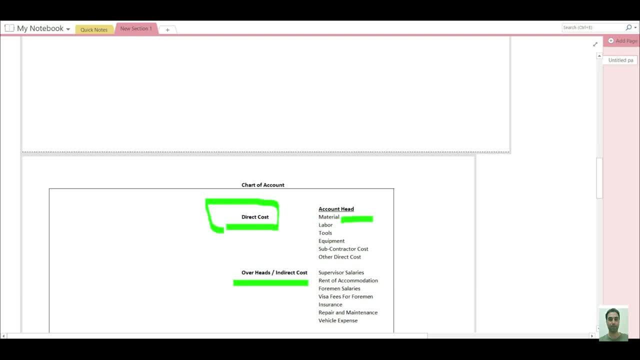 will assign here direct cost. in the direct cost you have material that has directly been used in that project. okay, now similarly, your labor cost is also being directly being used for that specific project. you have their time sheet so you can directly associate labor tools, then equipment. all these are the costs that are directly, that you can directly associate. 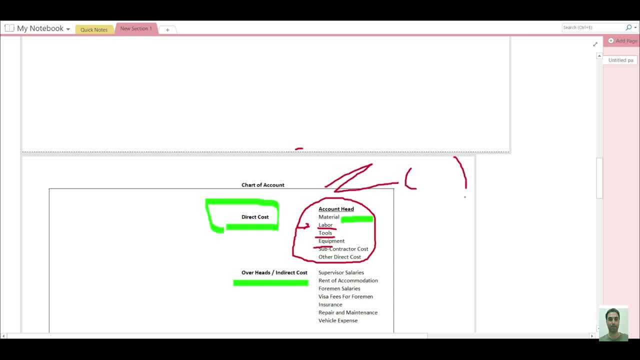 or directly charge to that project. here comes the concept of job costing. job costing means you are allocating the cost to those specific project which, though, that cost belongs to. okay, so this project, this material cost, is suppose material. you have stock room and you are issuing stock to different projects, so how much a specific material has been? 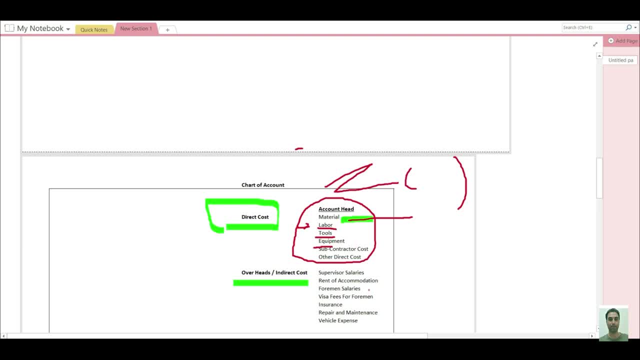 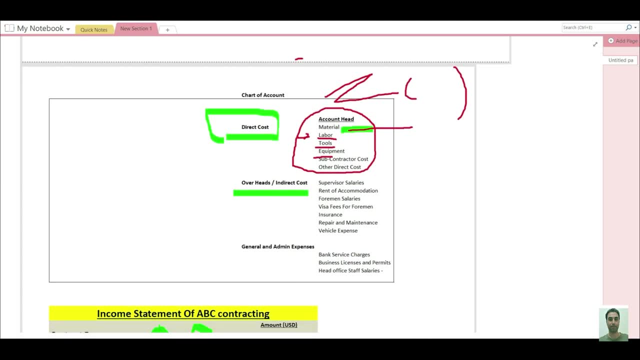 charged to specific project. you will easily know. so this is pretty much easy. as far as direct cost is concerned, you have different ways to trace it out. okay, but as far as indirect cost is concerned, i'm gonna tell you with an example. suppose what has indirect cost is concerned. suppose you have. 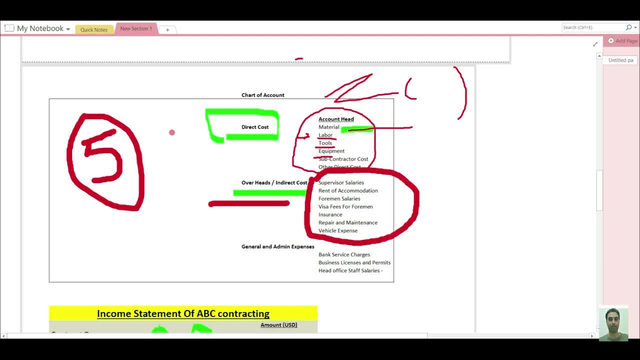 five projects, and those five projects are in same location. okay, but there are different projects. one is for, suppose, one is for, one is for road leveling, other is for epoxy flooring, other is for fire proofing or other sort of so. but but what happens it in the morning, your? 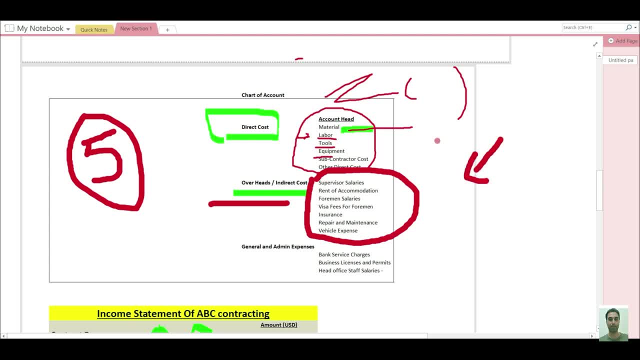 van or your vehicle took all the labors from your accommodation and brings them to these five location of these five projects. okay, so my question is: where would you charge the vehicle fuel for the vehicle that is bringing those labors to the sites for these five? your answer would be: this fuel or this vehicle is being used for the these five. 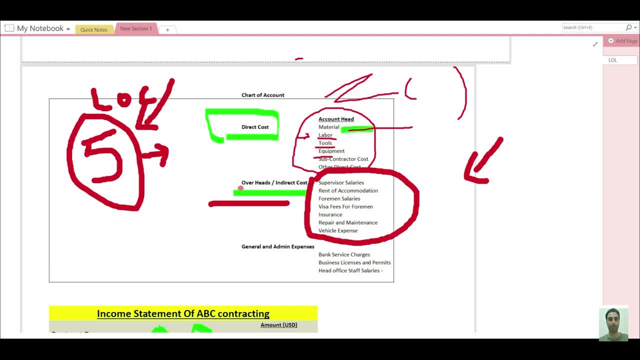 projects, but you cannot allocate them. you cannot allocate them specifically. so this is the no doubt, without the without vehicle being moved to that place and without the labors or foreman's being dropped to the specific location, they wouldn't have start the work. so this is of course. it is. 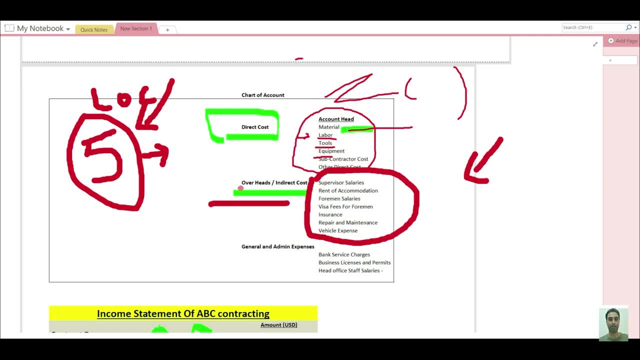 the cost of the contracts. this is the cost of projects. but you cannot directly allocate the cost of the contracts. you cannot directly allocate specifically how much to which project. so these are called overheads or indirect cost. you have got my point. so this is foreman salaries. 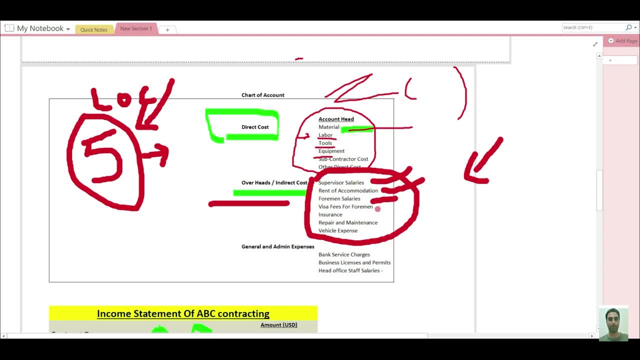 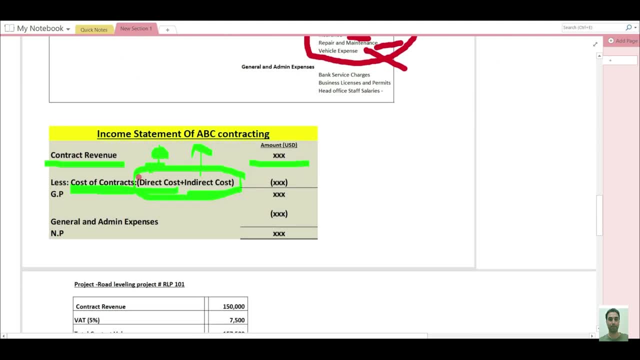 rent of accommodation for the labor where they are staying, foreman salaries, visa fee for insurance, maintenance and vehicle expense. so all these you will charge to them. so here, if you see that your contract cost- you saw the contract revenue- you will deduct cost of contracts or cost of project. 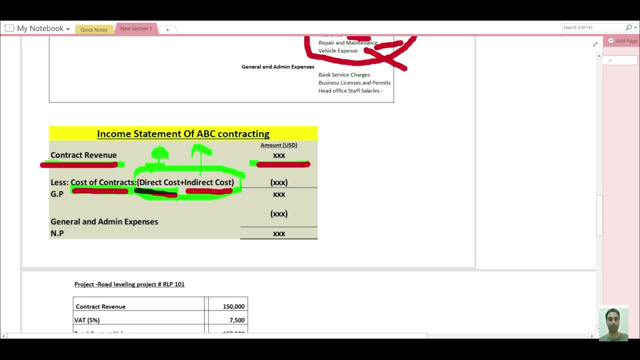 this cost of project is divided into two portion: direct cost and indirect cost, or you can say that direct cost or overhead cost. okay, so this- both overhead cost and direct cost- are both are what both are: your cost of contracts or cost of projects. after that, you will get gross profit. 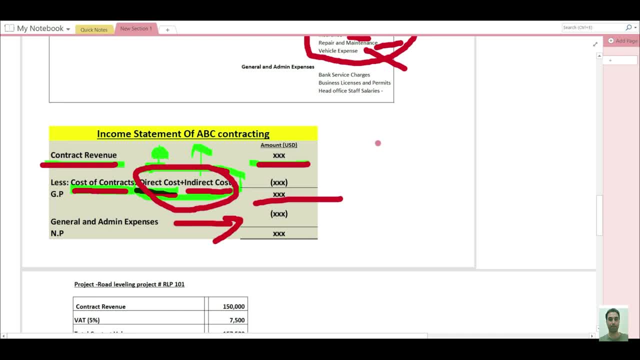 and then you will deduct from them the general and admin expenses. general and admin expenses are and the expenses like business services, business license permit, office and office staff, head office staff salaries and all these things that can that are not directly associated to the projects running. okay, so that's. 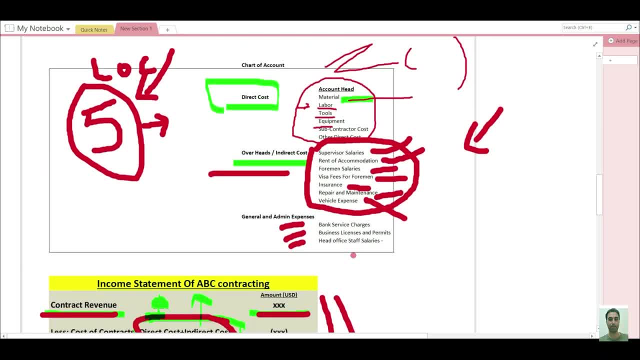 how it appears. one more thing that i want to show, tell you in the at this point is that as far as these indirect or overhead costs are concerned, you can allocate them to different projects by some professional way, on percentages or amount of time basis or pro databases you can allocate- suppose you have total. 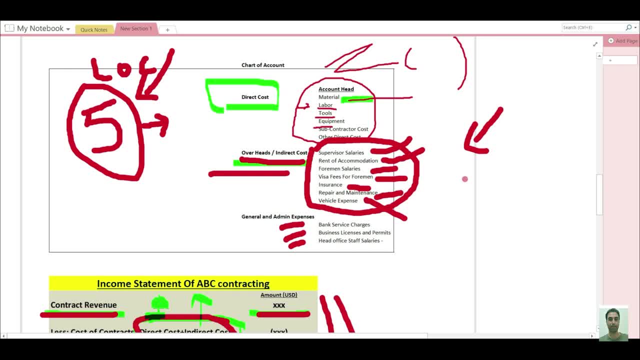 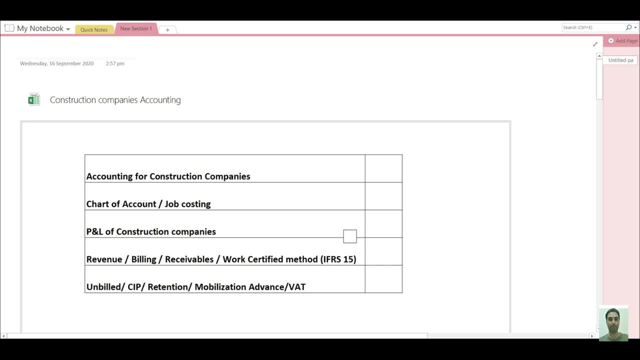 overhead cost for vehicle is 500. you can divide five. 500 divided by five is equal to 100 each project, and you can do that now. i'm going to discuss with you, with the help of an example, how you will implement all these things like revenue within a construction company. 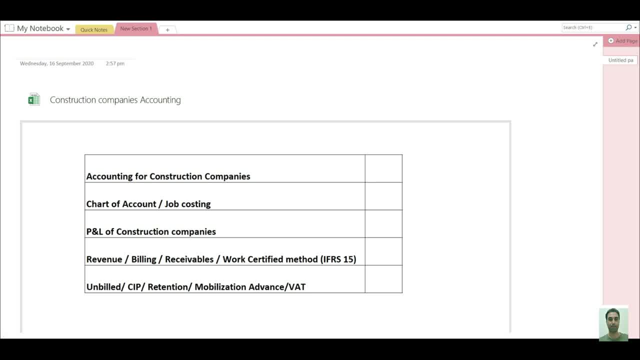 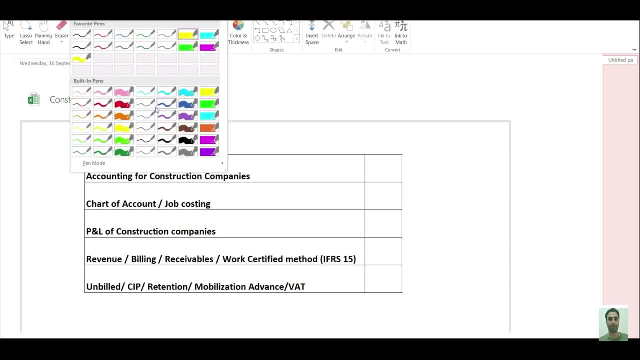 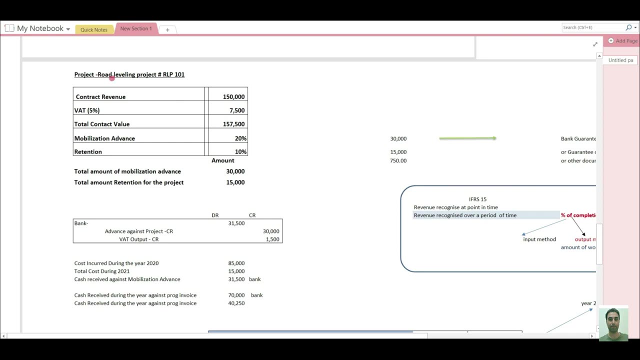 and after revenue, how you will deal with receivables, payables, invoices, how you will book the revenue and all this thing here. okay, so let's start with the help of an example. okay, suppose we have a project regarding road leveling and the contract value of that project. 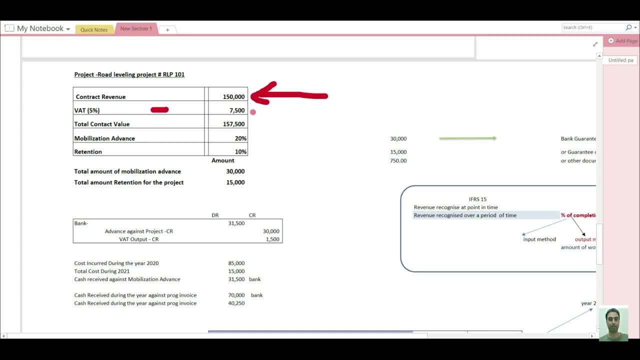 is one fifty thousand. that is five percent. so seven thousand five hundred will appear over here. total contract value would be one fifty seven thousand and the contract value of that project is five hundred. civilization is, advanced is twenty percent, retention is ten percent. okay, let me explain to you a little bit more about mode, mobilization, advance and retention. okay, 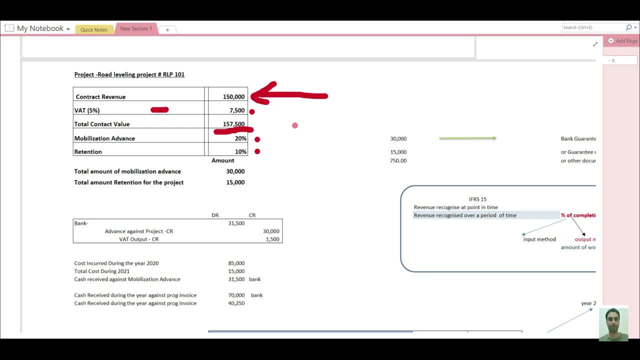 mobilization advance. twenty percent means you will get twenty percent of the project upfront, the amount of the project upfront and this twenty percent will be detected from each progressive invoice. same percentage: this is how mobilization advance works. okay, now i will discuss with you retention. retention is the amount which has which will be retained from each progressive invoice at the rate. 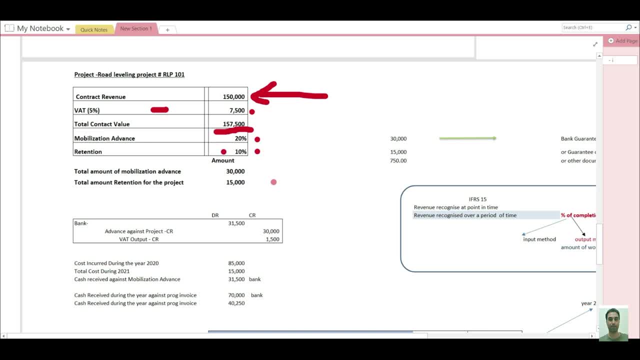 of 10 percent in our example, and it will be paid to you after the completion of the project. that's normally it, that that is normally how it works, okay. so as far as this mobilization advance is concerned- in our case it is 30 000- what happens is that sometime, because they are giving you 30, 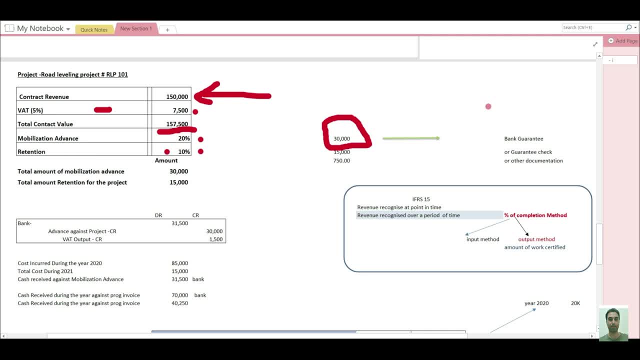 percent in advance without doing or performing any work. so the company, those who are giving it to you, they provide, they ask you for some bank guarantee or check or any other documentation as far as their need is concerned or your contract is concerned. so in this, in our case, total mobilization advance is 30 000, without 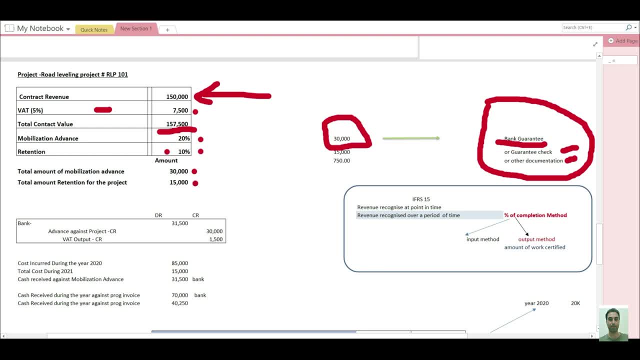 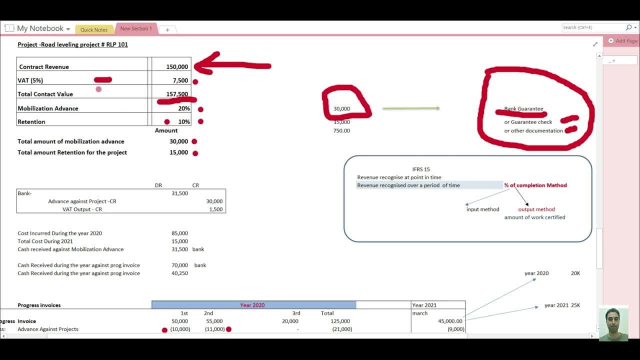 okay, so let's start and do how we will proceed. so now just look at that and then we will bring, then we will begin. okay, so we have this project. let's start this project, working out as if you are working in practical life. okay, so now you have got this project, what will happen? you have 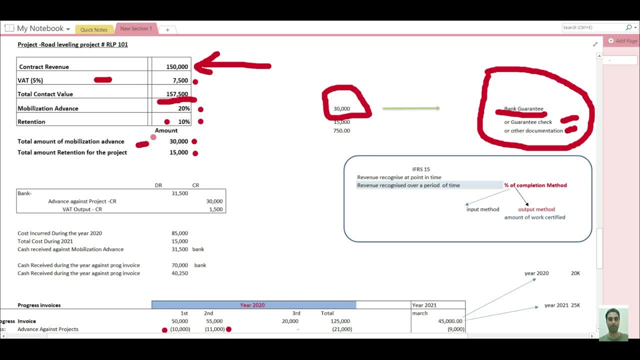 now. the first step is: you have received your mobilization advance of 30 000. okay, you have received your mobilization advance for this project and we have received your minimum of 30,000 here. if you see over here now, you, what will happen? your bank. 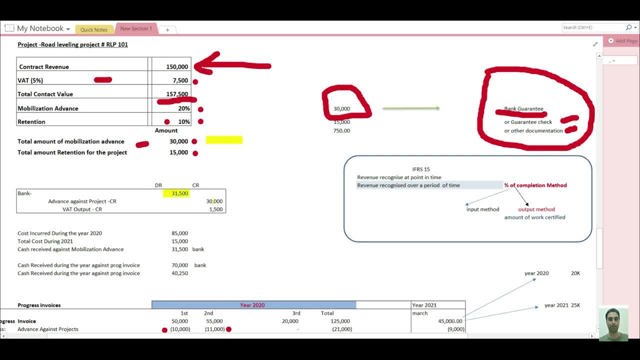 account will be debit. if you're in the bank account, you will get 31,500. why? because 5% is the VAT. also, you received same 30,000 you have received as liability against your project. because why, but you? what will you do? you will. 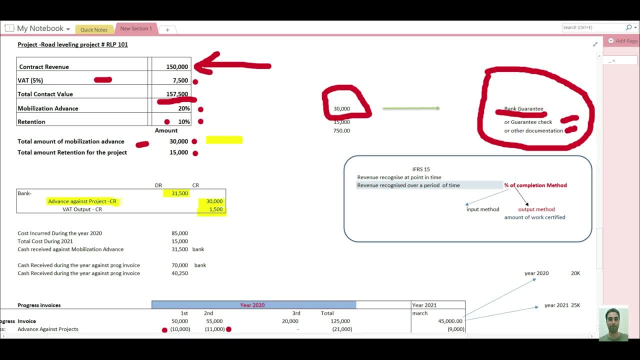 debit bank. you will put 31,500 in your bank and what you will credit? you will credit advance against project, advance against project. you will credit because, why? because this amount, this 30,000, you against this 30,000, you have not performed any work. this is your unearned income. so this is the general entry and 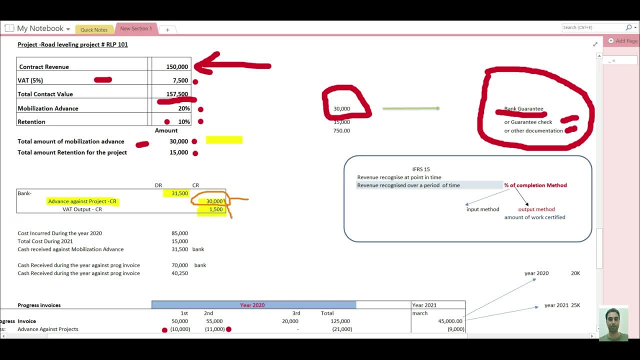 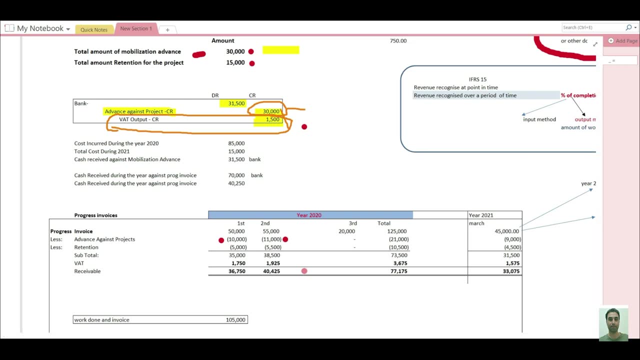 as this. as far as five percent retention is concerned, this one, this is your VAT output liability. so you, you will just take from the client and pay it to the government. you have received initially advance and 31,500. that 31,500 has to be. this is your bank and this is your advance. this is your VAT. okay, now after. 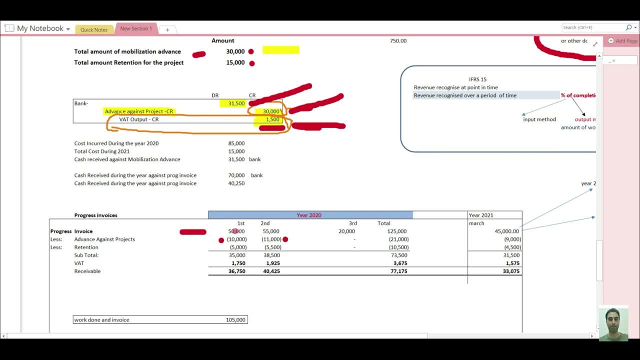 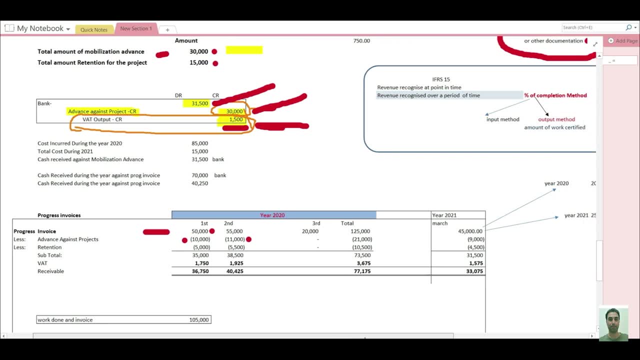 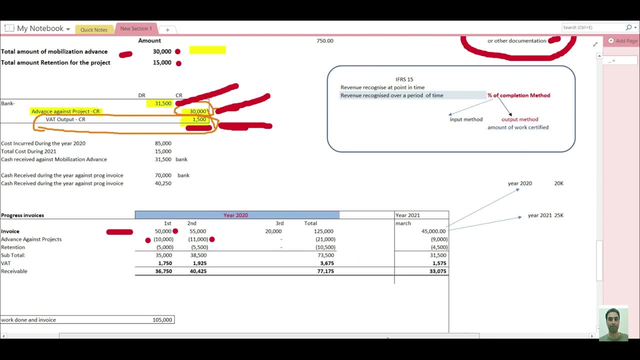 three months you have performed the work of 50,000. if you see over here, this is your first invoice: 50,000. okay, now, at that time, I want to discuss with you the concept of revenue. so you will. you have performed work of 50,000. okay, now before. 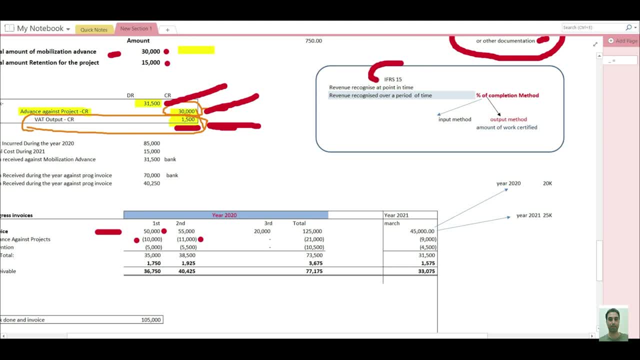 going to that. I want to explain to you a little more. as for IFRS 15 is concerned, IFRS 15 says that you can recognize the revenue as far as contract revenues are concerned, revenue at a point in time or over a period of time. so this is not none of our business over here we are. 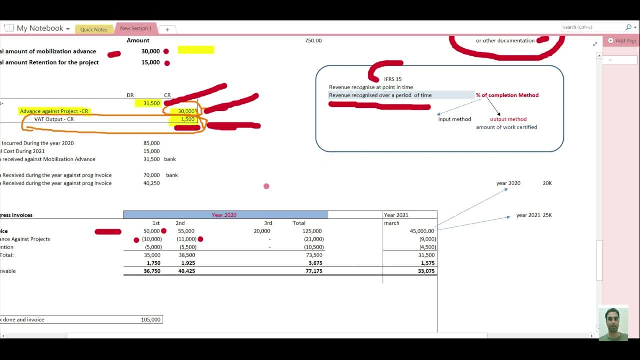 dealing over a period of time? okay, because it this project prolongs to two years, to year 2020 and year 2021. okay, then you are recognizing the revenue over a period of time. IFRS 15 says that we can make it on basis of percentage of. 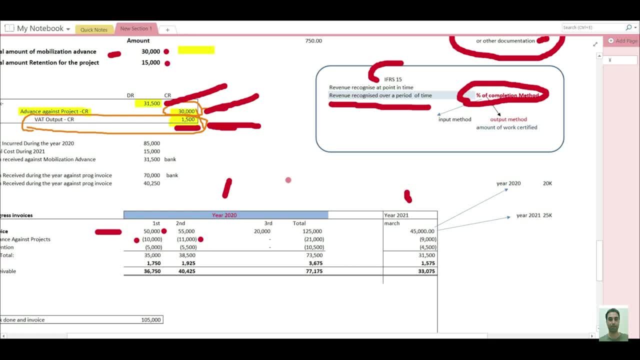 completion. what percentage has been, what percentage of work we have performed and we can book revenue. as for that percentage of completion, okay, in the percentage of completion we have two methods. one is output method, one is input method and the input method. the focus is on how much cost that we have. 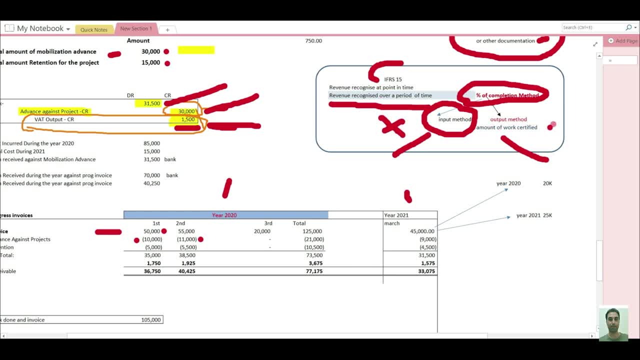 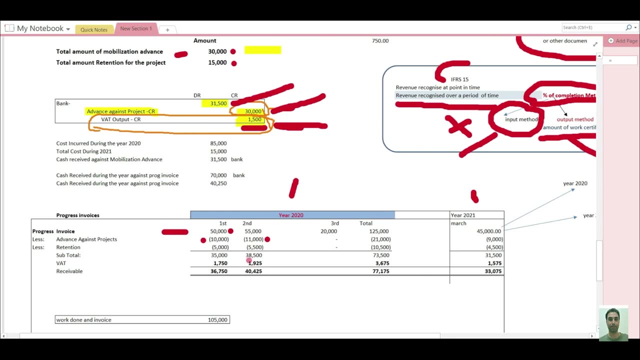 incurred. we are not using input method over here. we are using output method. output method focus on how much work we have produced or output we have produced. we are using output method over here and the output method. we are using work certified we have worked performed up to and we are assuming that we- I am not- 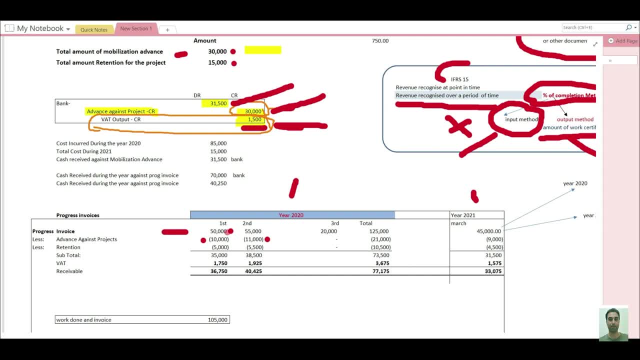 making things complicated here, that, okay, we have performed the work of 50 000, but we have built 40 000. so no, I'm making the things simple and I I will suggest you. you should also keep the thing simple, however, if it is unavoid, unavoidable for you. 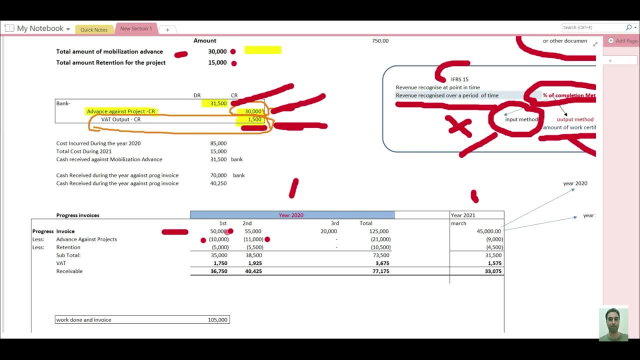 you can go and watch my video on output method and that method. there is difference between how much we are invising and how much we are actually performing the work. but here I I will recommend you you should use this method that I am using over here in this example that, whatever work you are doing, 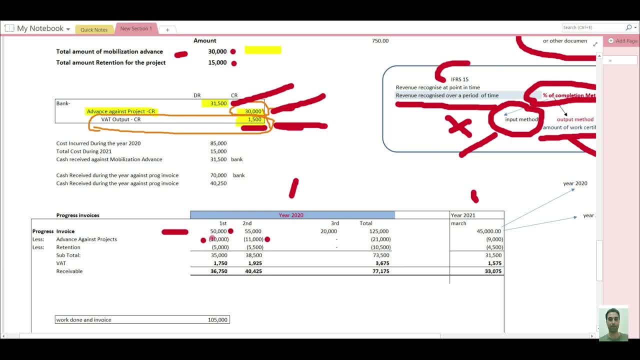 you are invising. so I have performed the work of, as per my engineer. as for my surveyor, I have performed the work of 50 000, so I will invoice them 50 000, but wait for this 50,000, for this 50,000, we have retention, we have advance against project, we 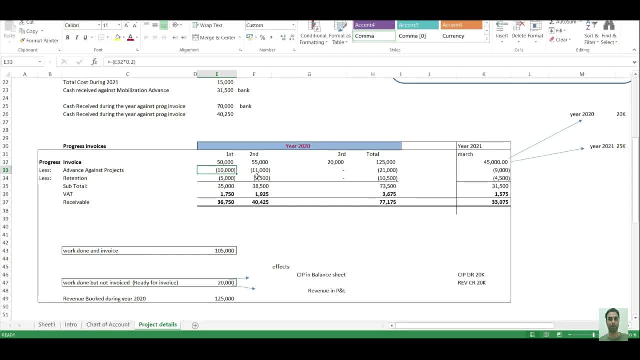 have VAT. how we will deal with that. we have this 50,000 now. in this 50,000 we have 20 percent advance. we will deduct this 20 percent advance from this 50,000 and then we will deduct 10 percent retention from this 50,000 and the net amount will be 35,000. from this 35,000 we have to apply. 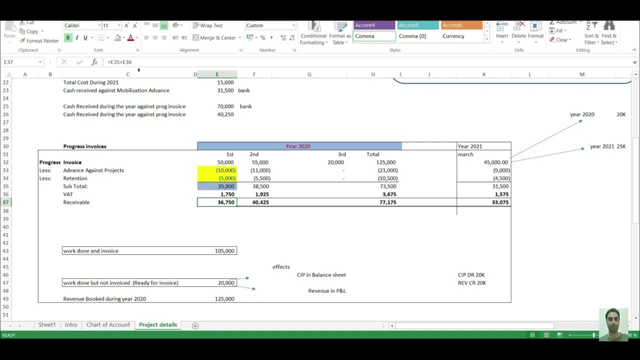 VAT on this, that is five percent, and net receivable, including the VAT after the retention, after the advance reduction, is 36,750. now, if you have any question regarding what about the VAT on retention and what about the VAT on this advance against project, why we are not putting VAT on this 50,000, the answer is: as far as this advance against project. 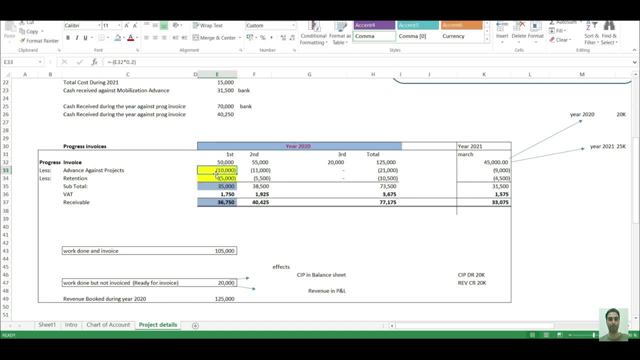 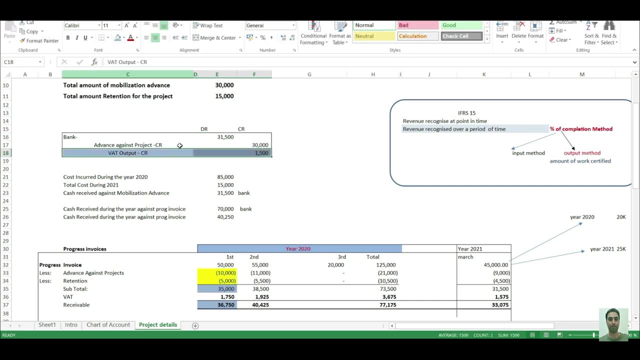 or this advance, that 31,500 is concerned, it is charged at that time. we receive 31,500, so this VAT output has already been charged on it, so we will not double charge it, okay. so that's why I have reduced this amount, this 10,000, which is a 20 percent of this amount, which is a 20 percent of 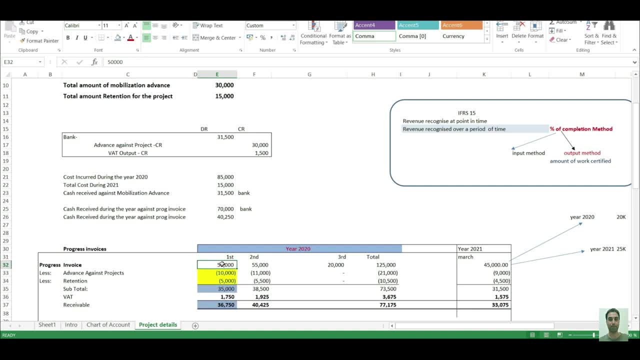 one more thing: you to not reduce all this 30 000 from first invoice. this is not what usually happens in contracting or construction companies. they have some rules like 20 percent, 30 percent, 15 percent. they give you the project 15 percent, 20 percent amount advance, amount of advance from. 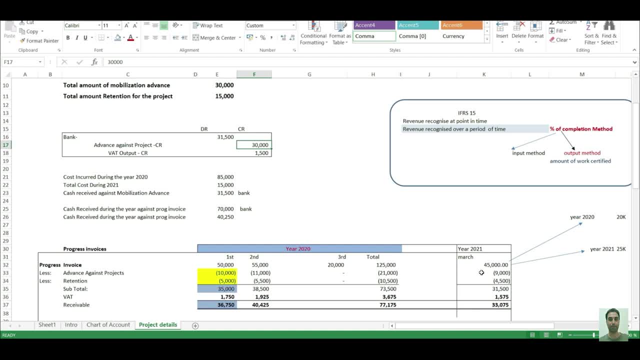 the project, and then they reduce with each progressive invoices. okay, okay, now that's why i have reduced this amount 10 000. as far as retention is concerned, the rule is that whenever you receive the actual amount of retention, at that time you have to charge VAT. 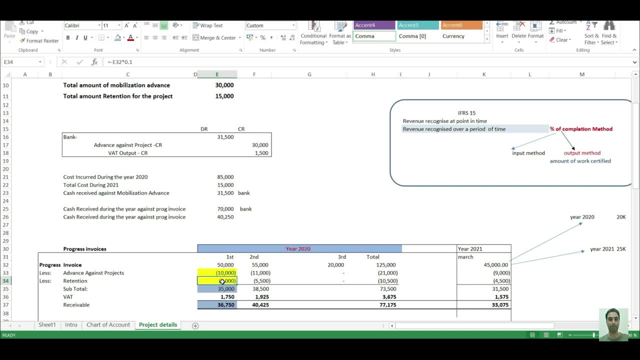 or when you invoice for retention at that time. whichever is earlier, you have to charge VAT at that time. so here, in this case, we are neither receiving the retention amount nor we are invoicing the retention amount. we are just deducting here. so that's why i am not considering it. okay, anyway, don't forget, don't bother a lot. 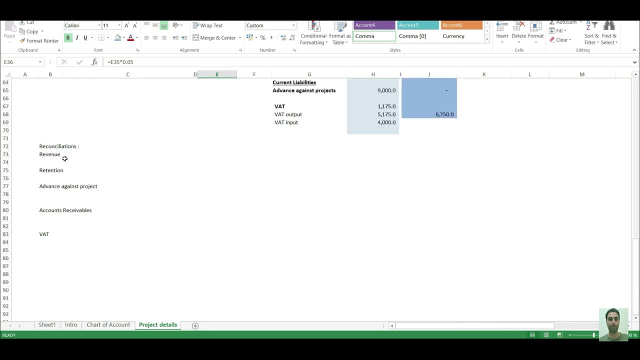 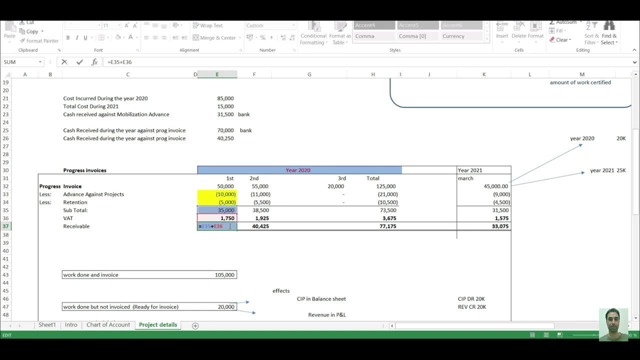 about this VAT thing. i will do reconciliation, that- how much total VAT has been done at that and once we will finish it. okay, okay, so this is a total amount of the invoice that we have given them after the end of three months, when we have, once we have performed the work, right. 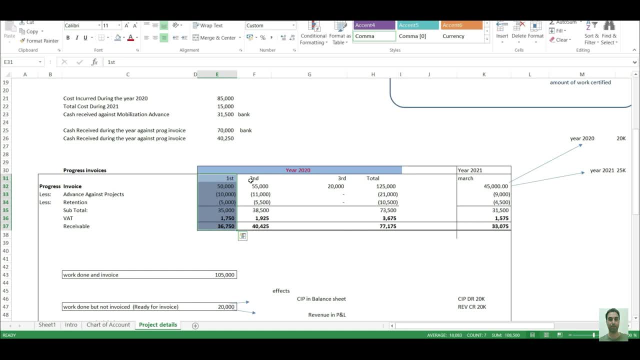 i hope this is clear for you. okay, three months have passed. we sent them this, and after that we have sent them a second invoice and the till the second invoice, we have performed the work of for the for that, the third period for from them. then we we have performed the work of fifty five thousand. 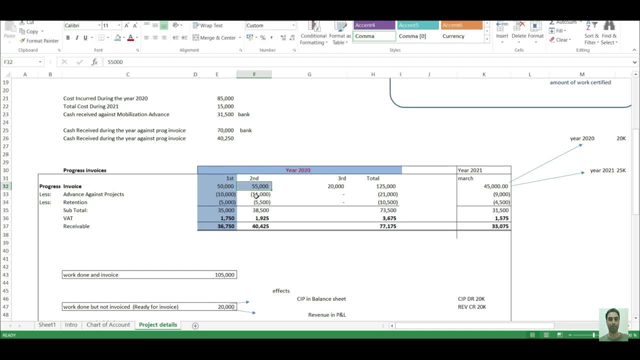 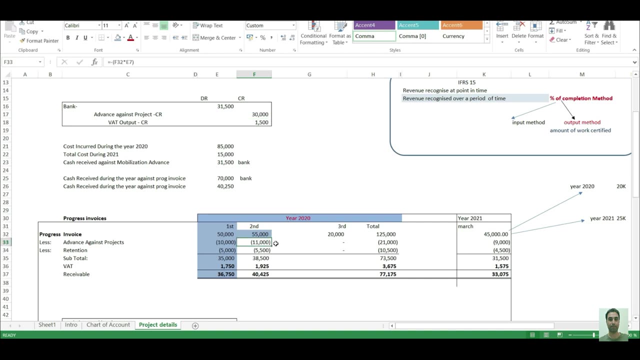 bear in mind. this is apart from that. after that, this is the second invoice. for fifty five thousand, again, same thing will apply. twenty percent, we will reduce deducted, and our balance of this amount, this thirty thousand, will be reduced with minus ten thousand, minus eleven thousand, so and so total. 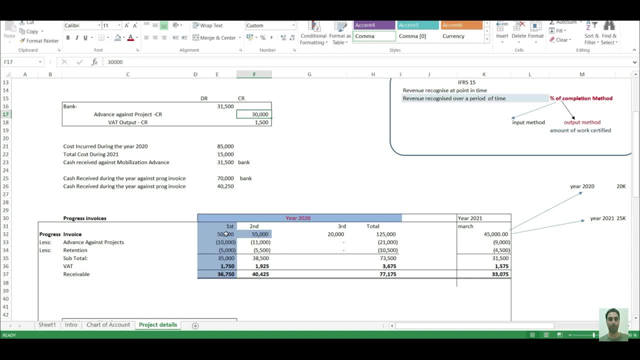 amount is how much? now, twenty one thousand. so thirty thousand minus twenty one thousand nine thousand will be your remaining balance after the end of second invoice. okay, all right now. what next next? let's same way happen with the. what is this retention? this is your retention. let me color it something in, so you should know: this is to your retention, this is your. 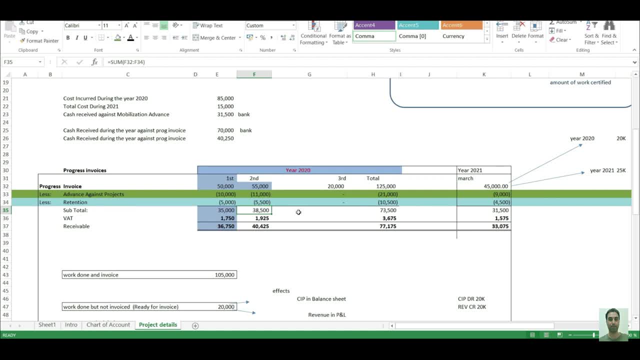 advance. okay, all right. so now this thirty eight thousand five hundred. we have applied the vat on this thirty eight thousand five hundred and we have sent them invoice. this is the receivable net, receivable from progressive invoices. okay, all right. so these two things are done now. now let me discuss with you how the effect of these 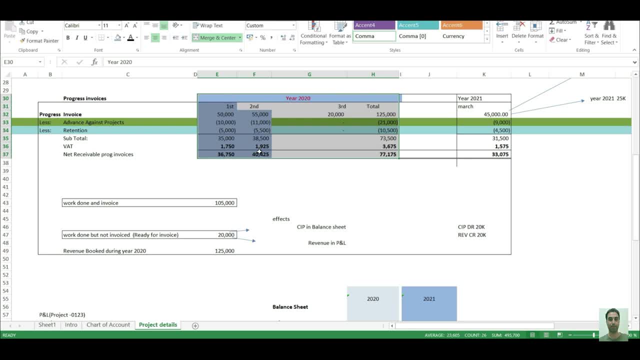 invoices will goes to financial statement, pnl or balance sheet. the effect of this fifty thousand will goes to your profit and last count income statement. this will go to your profit loss income statement, as far as this is concerned, where it will go. as far as this is concerned, where it will go. 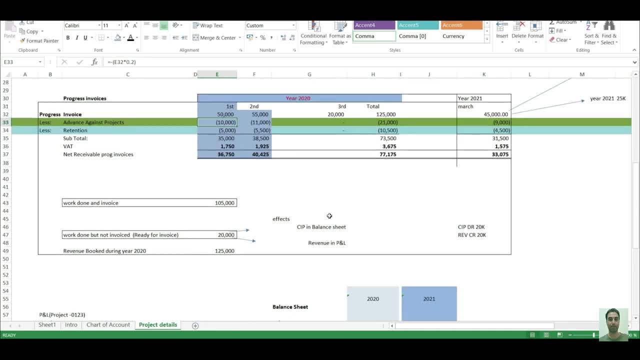 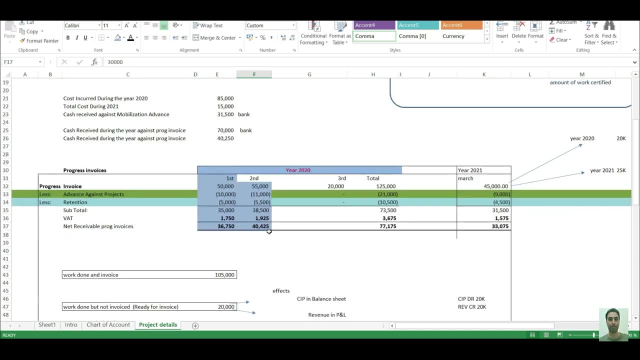 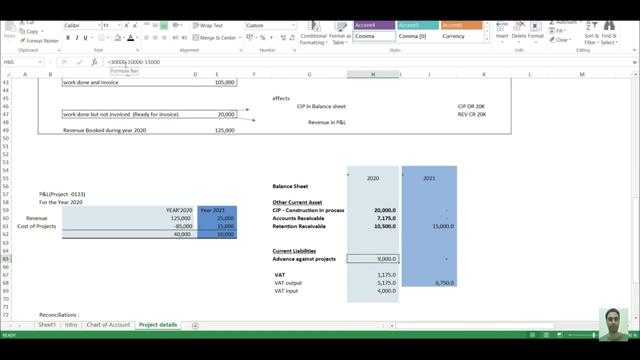 this will goes to your balance sheet. first you will book this as a liability of thirty thousand, then this amount will be reduced from this liability, and then this amount will be reduced from this liability. so your net figure at the end of the month will be this thirty thousand. 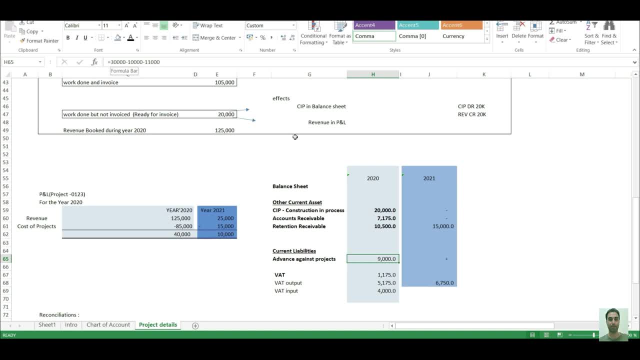 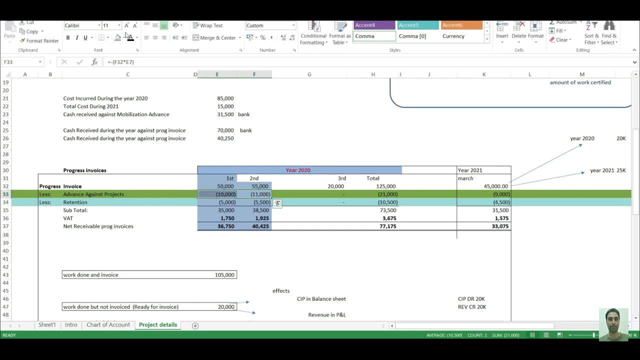 minus ten thousand with the first invoice, minus eleven thousand with the second invoice. so this will be your net figure after doing all this. okay, this is done, these two are done, these two will go to the pnl. okay, and the fact of this retention, now, as far as retention is, 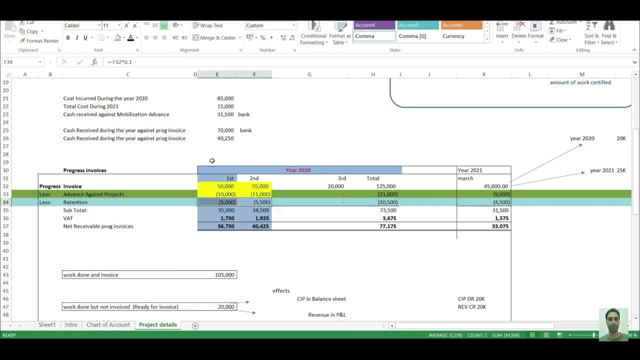 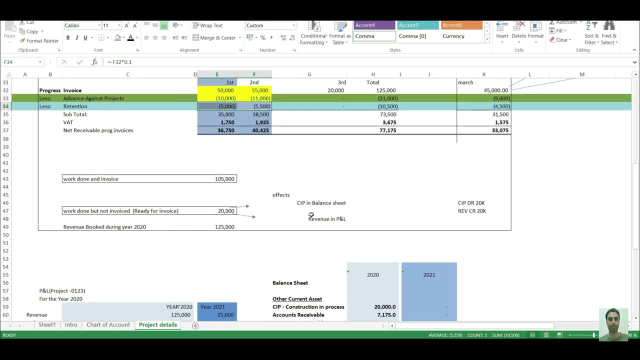 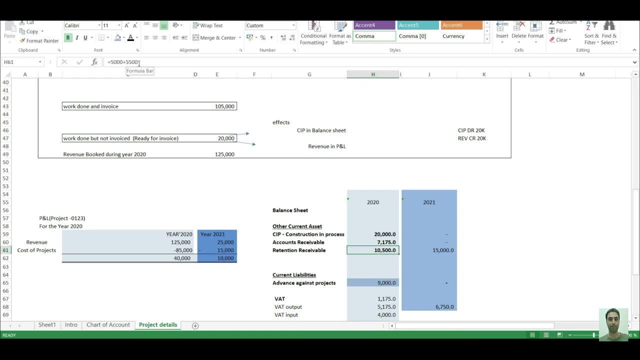 concerned. this is just your receivable. only the time is delayed, so this you will book separately. retention receivable as this amount 5 000 plus 5 500. where is the retention? yeah here, 5 000 with the first invoice and five thousand five hundred with the second invoice. so this is your return. 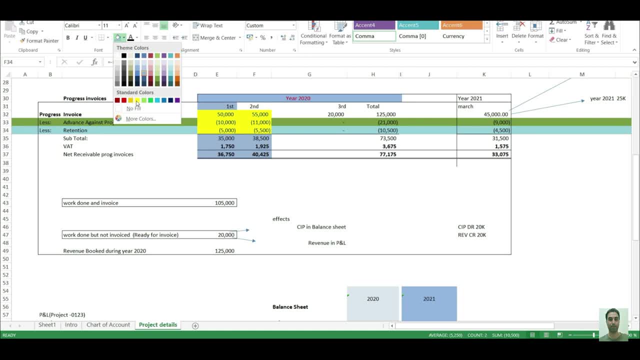 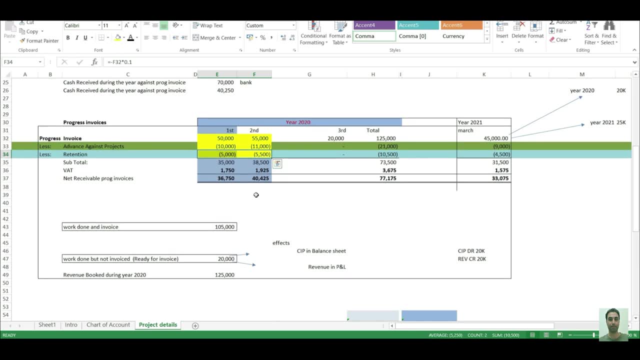 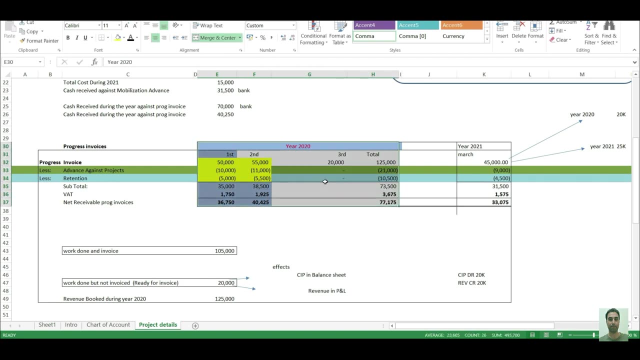 clear now. okay, all right. now there is another thing that i wanted to discuss. i have deliberately did this so you could know this concept as well. now your year 2020 has end, but you have not advised the customer. again, i will say so you can listen to me: your year has ended, but you have not. 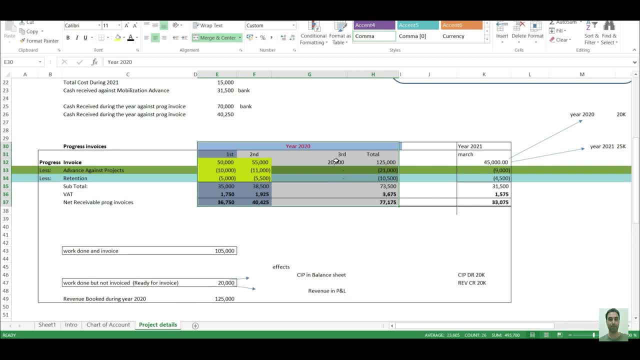 advised to the customer. but you have performed a work of twenty thousand as per as your engineer or surveyor or your work in charge is concerned. you have performed the work of twenty thousand. then what will you do? as far as output method of concern, you have to record. 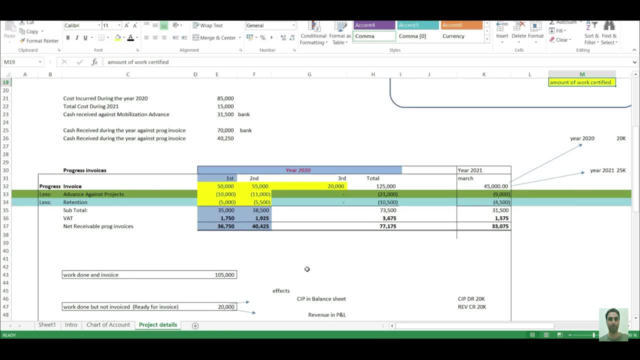 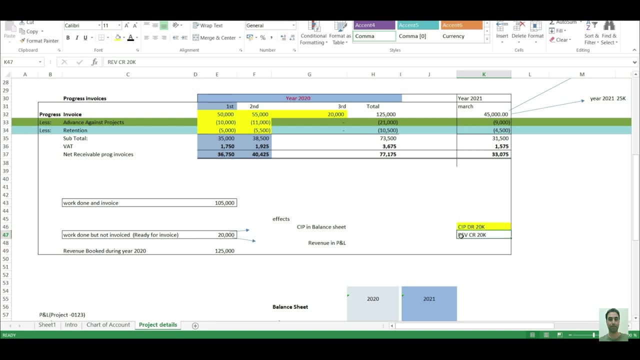 this twenty thousand as your revenue. okay. so what you will do? you will debit construction and process, debit the account with twenty thousand and credit what revenue with twenty thousand. so your total revenue for the year 2021- 2020 will be one thousand twenty five thousand. why this? this plus this, okay, but as 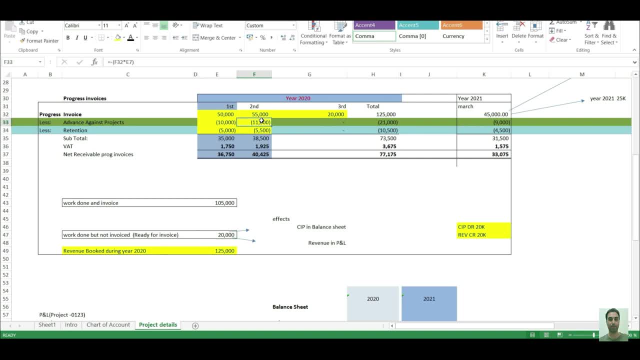 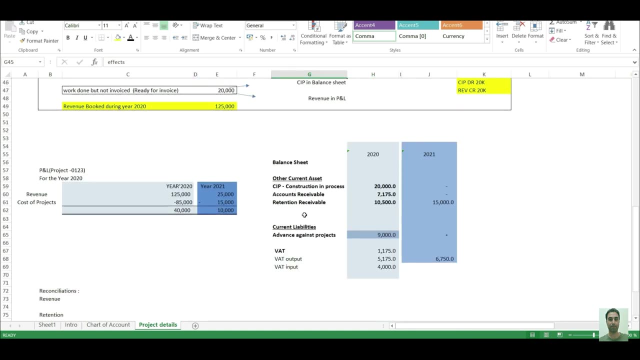 far as retention is concerned, as far as uh advanced against project is concerned, you will not deal with that, because this has this, this, this deals with once you will invoice the client. okay, okay, so you will do this entry. all right. now let's see how these will be presented in year 2020. 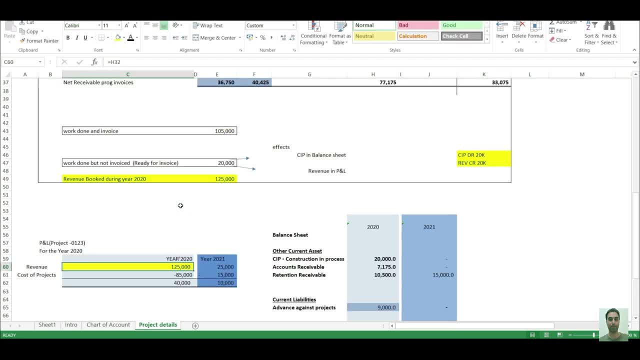 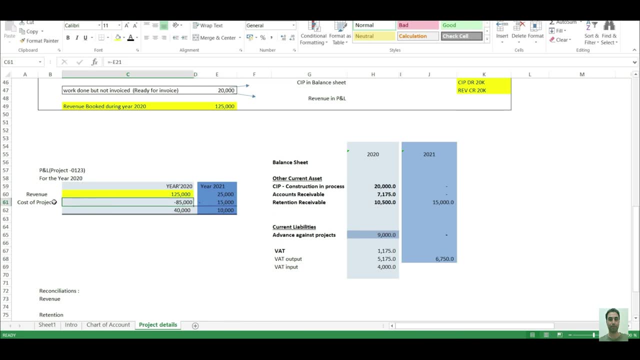 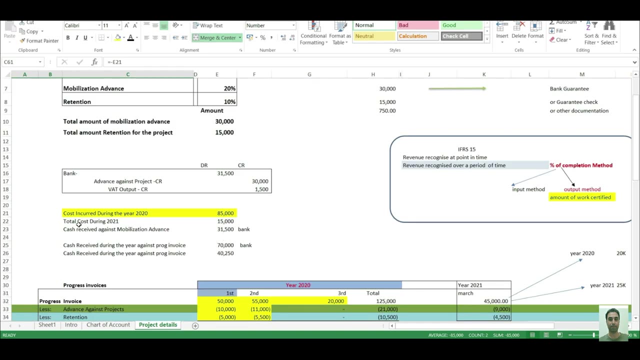 here, 2020, your total revenue is 125 000 and i see here: total cost incurred for the year 2020 is 85 000. you will just write cost and you can just job cost them according to your projects and whatever. okay, all right, then let's see total cost. okay, mobilization at. 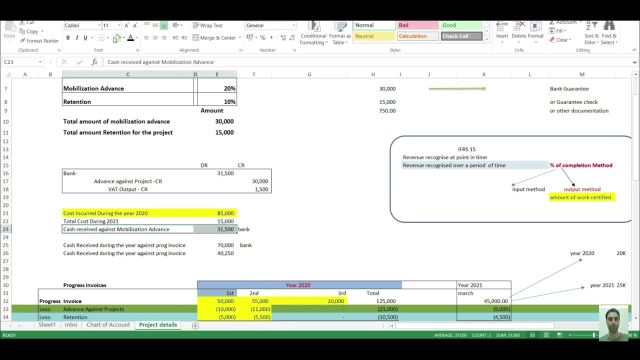 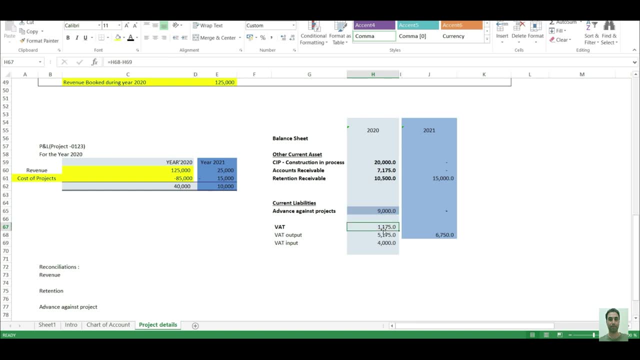 once have. we have done it. um, okay, the effect of this mobilization advance, we can see it here. this mobilization, 30 000 come over here and that, uh, as far as that output is concerned, this fifteen thousand you will add over here as a wet output. okay, this fifteen thousand, now your weight is 1500. 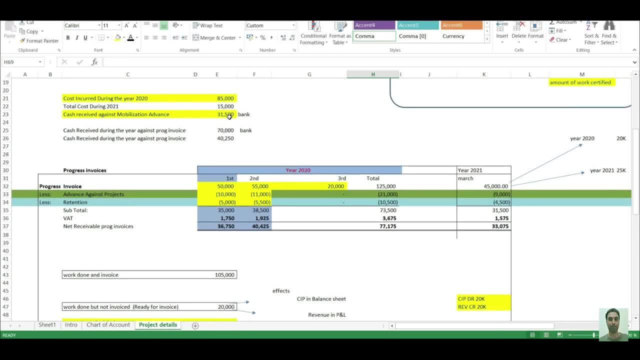 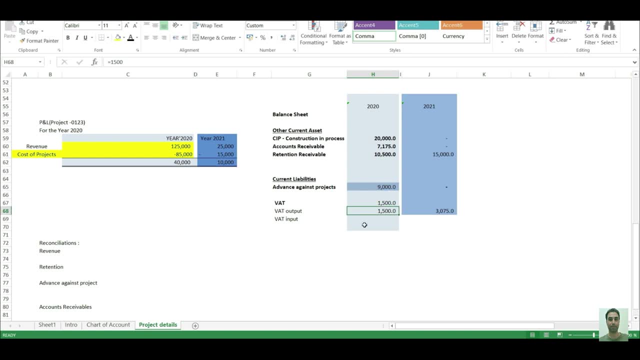 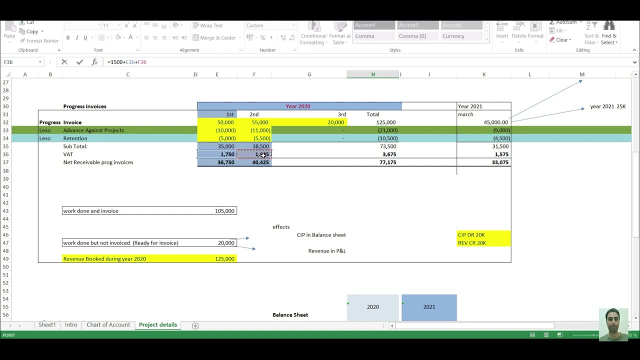 okay, where does this fifteen hundred can actually be put over here. the output is 50 000 and we have a output of 500 000. so this is the utility in this unit. so the utility is here here. mobilization advance has wet for the year 2020, so you will write here that output as 1500 plus. you have charged them that with the. 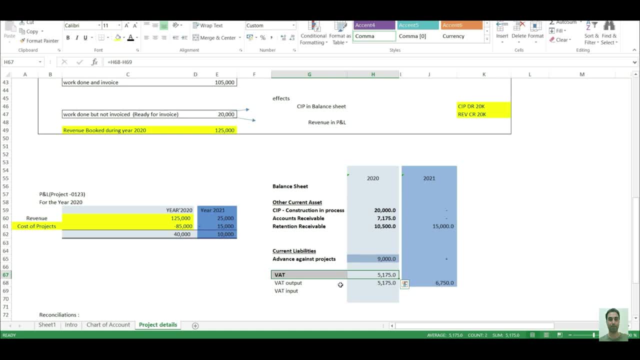 worst progressive invoice plus second progress of invoice. so this is how your it will appear back. okay, okay, one more thing i wanted to tell you over here is that your liability or refund, so it net amount or VAT control amount will be shown over here. but for the sake of understanding you are telling you I have done it like we assume. 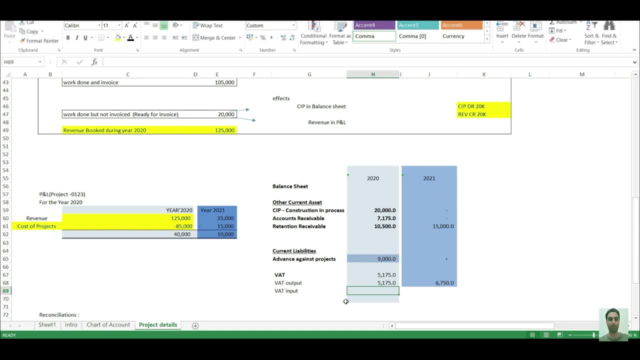 that you have VAT. this 85000 is equal to 85000 into 5%. so this is your VAT input, VAT output minus VAT input. so your VAT liability for this year would be like this: okay, this is how it came over here, all right, I hope you understand this concept now. this year has 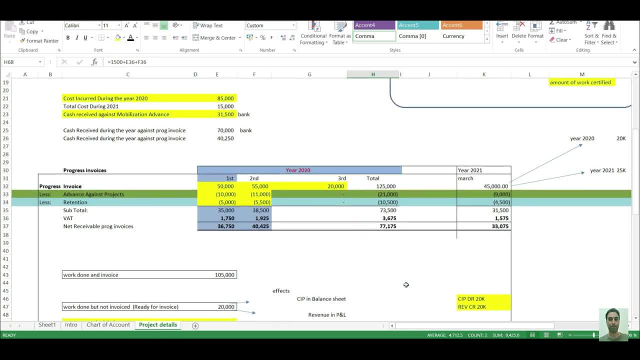 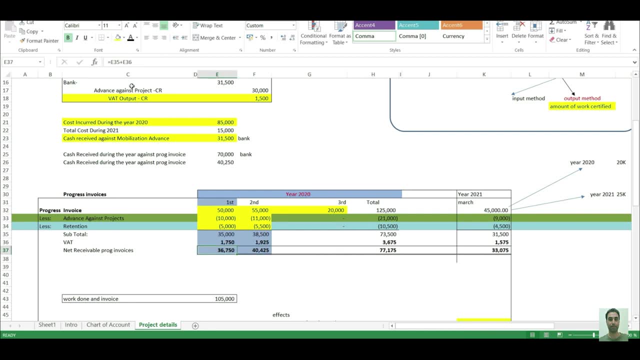 ended. no one more thing. what is one more thing? yeah, yeah, the other thing that I wanted to tell you is receivable. so you have booked the receivable here from here. this is your receivable. you have, you are booking receivable from here: 36000 plus 42500. okay, this is what. 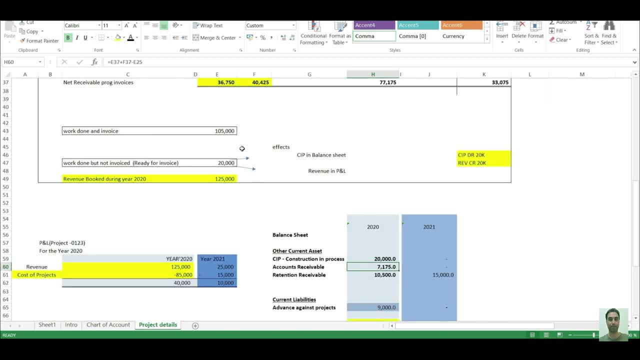 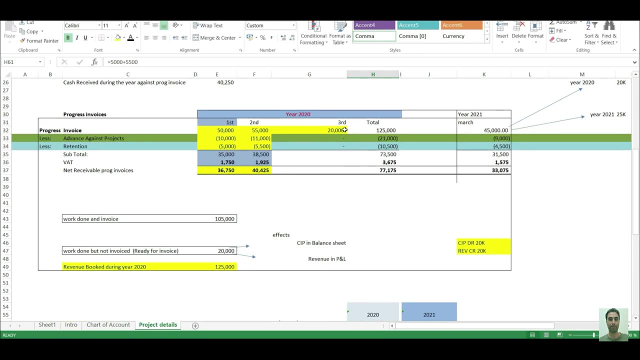 you have booked the receivable. so where are you receivables? your receivables are here, these two. okay, so your receivable is equal to this plus this. okay, again, i'm gonna tell you you will not book this receivable. what you are doing, you are debiting cip, debit and revenue. you. 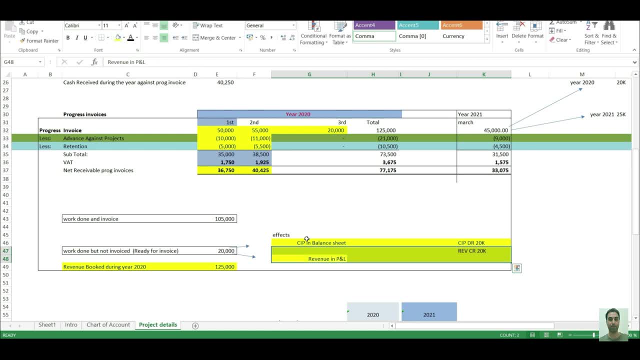 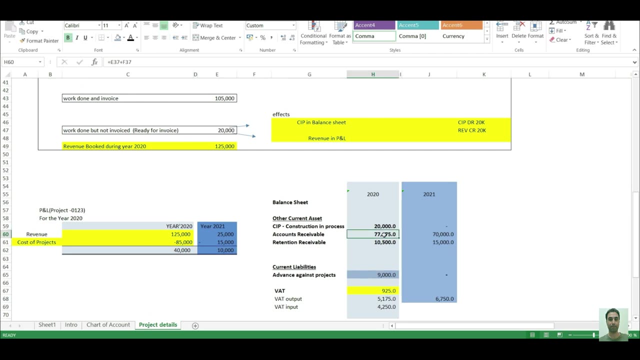 are creating with the same amount. we're not booking the receivable. against this advice. okay, against this 20,000. what is this 20,000? this 20,000 is the amount of work done but not invoiced. okay, so this is a kind of unbilled amount. okay, okay, this is 77,500 minus how much you have. 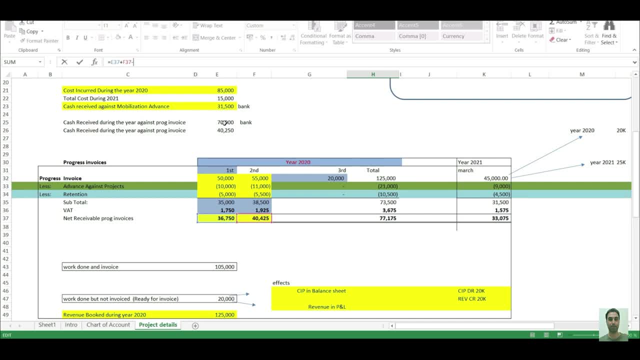 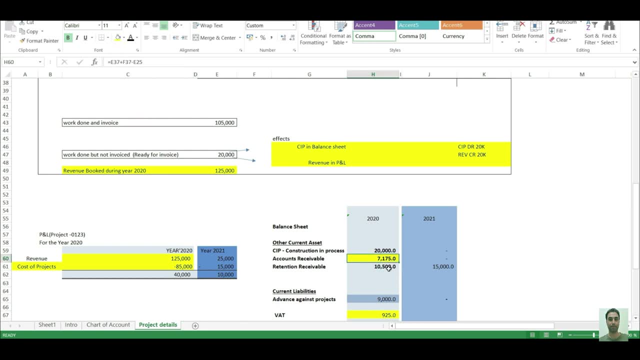 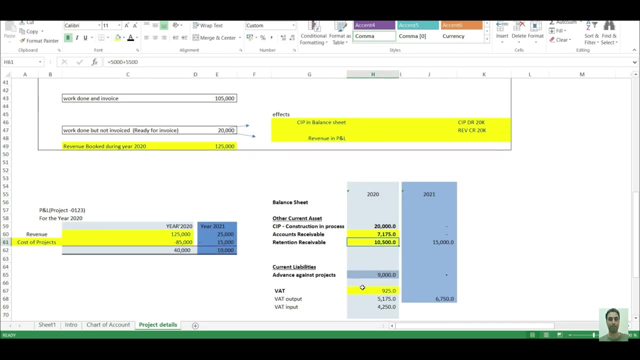 received against progressive invoice during the year. you have received 70,000, so this would appear. so we have discussed this done. we have retention receivable. as far as retention receivable is concerned, this plus this, you will just enter here in the balance sheet. okay, advance against projects. we have done. 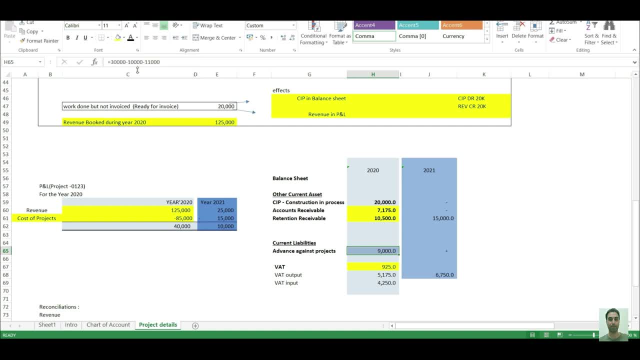 it. 30,000 was your advance against project. 10,000 is adjusted from invoice number one. 11,000 is adjusted from invoice number two. okay, as far as that, till end 2020. whatever done, i have adjusted as far as this construction and process, as far as this will appear in other current asset here: okay. 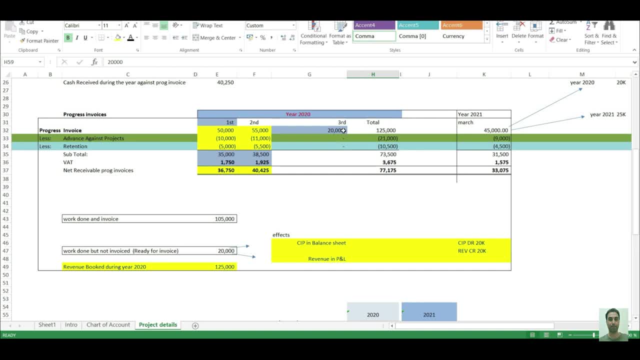 this 20,000? where? where does this 20,000 come from? this 20,000? this is debiting the CIP with 20,000 and correcting your revenue with 20,000. okay, this is work done, but not yet invoiced. 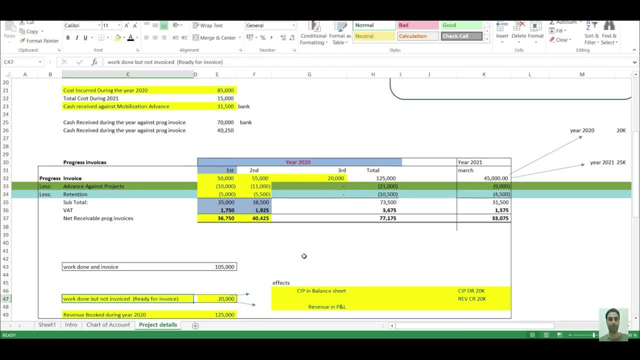 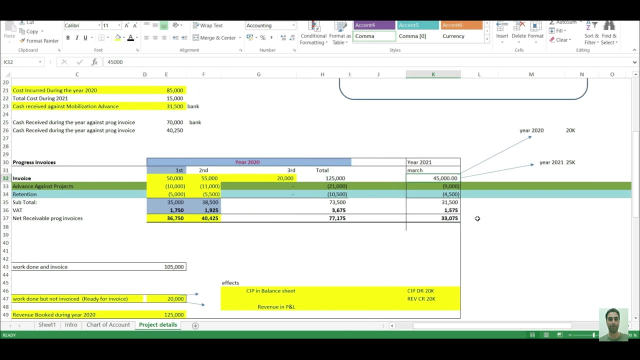 all right now. year 2020 has finished. stay with me. it is very important. what will you do in year 20, 21, once you will invoice this 45,000, including the work of this 20,000? okay, now, in the year 2021, you. 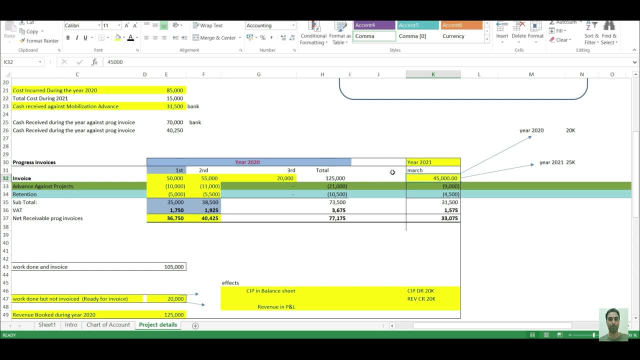 have invoiced 45,000. now this 45,000 includes the amount of 20,000. okay, so what I will suggest you is that just invoice 45,000, simple, and their effect will automatically go. revenue will be credited, output will be credited. that output will be credited and what will happen? account. 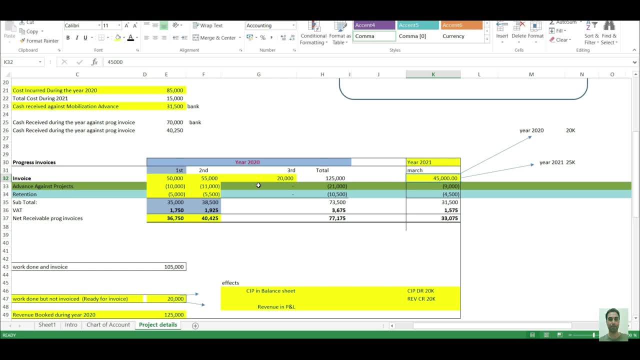 receiver will debit. okay, he will say: yes, sir, I listen to you, but what happens is that I have already booked my revenue- 20,000, and year 2020- once I will book this, 45,000. my total revenue that I book will be this plus this, so this is 170,000. however, I have performed the work of 150,000 only. 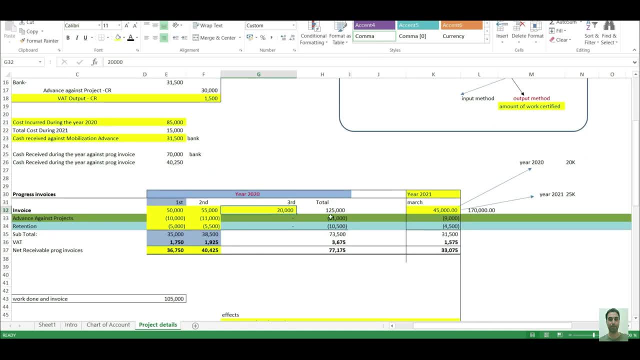 my project is 150,000. so what will I do with this 20,000? I will say: just do a simple thing, just make the reversal of this simple. at the same date, when you will book this 45,000, what will happen? the effect will be: 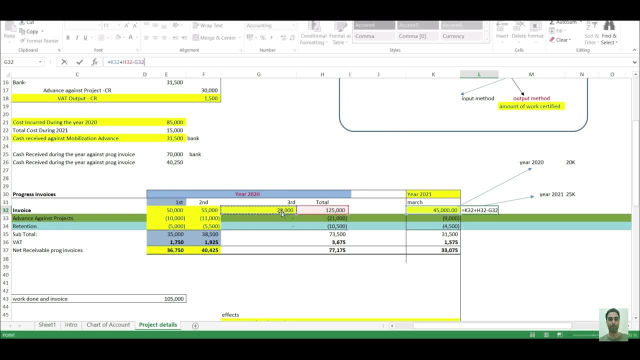 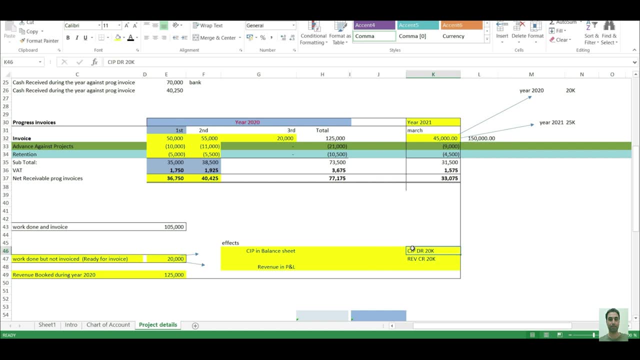 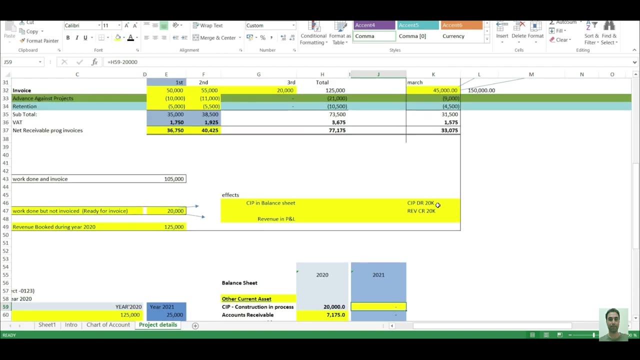 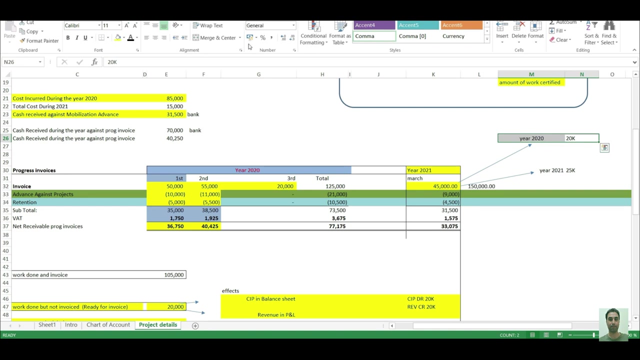 my minus 20,000. so what will be the general entry for that? debit CIP, debit revenue with 20,000 and credit CIP? CIP will be removed in the year 2021 and what will happen? revenue will be reduced in 2021 with 25, with 20,000. so what, effectively, you are doing? you are booking revenue from this. 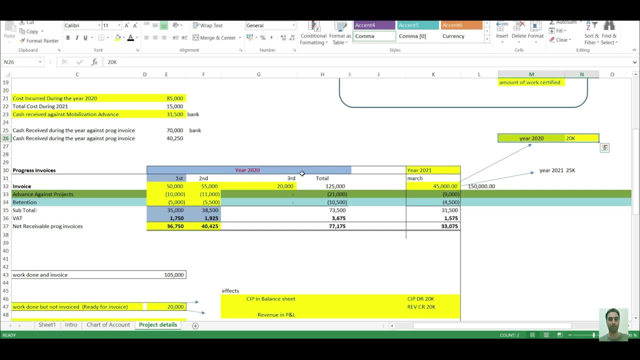 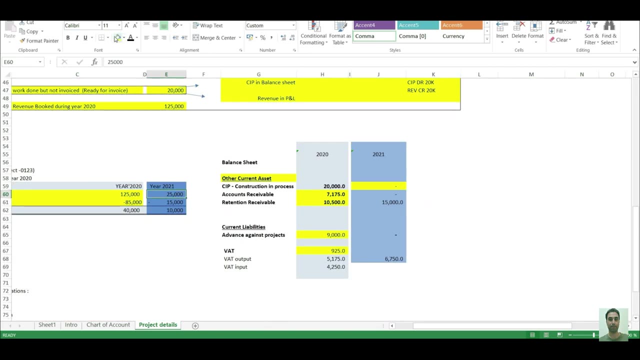 45,000. you are booking 20k in the year 2020.. and 25k in the year 2021.. okay, so I hope you understand this concept now. it is very easy for you. in the year 2021, you will book how much your revenue will be here. 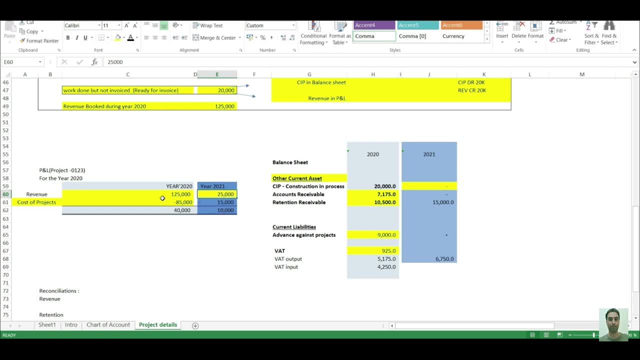 though you have, though you have invoiced them 45,000, but how much revenue will be in your P&L 25,000? why? because of reversal entry, you will of 20,000, so 25,000 minus this year. you have this much cost remaining this, so that is how it will. 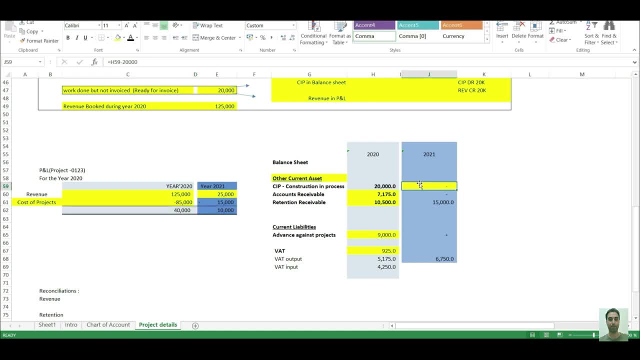 appear. so let's see one by one, construction process. you understood why: because because of reversal entry, it has disappeared. as far as receivable is concerned, let's see what happens to receivable. so you have had this seven in the year. you have this, let's do it now- is equal to. 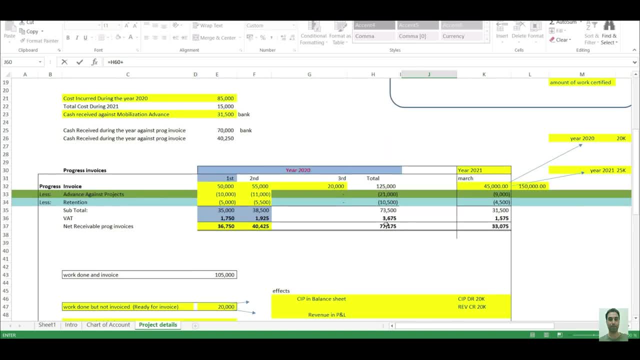 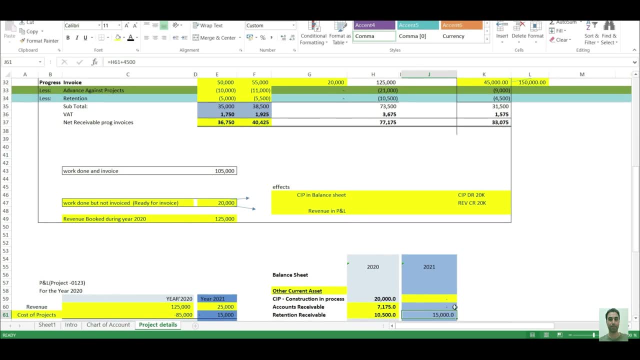 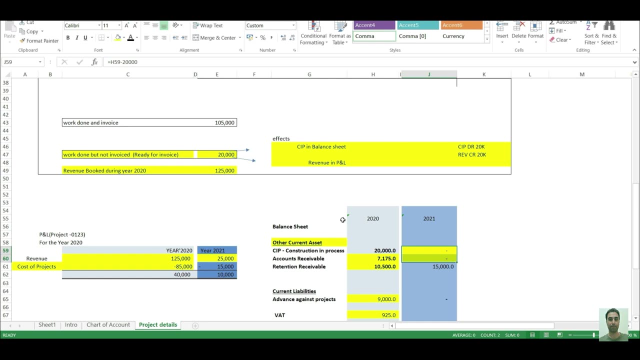 this much you have opening balance plus, and this year you have booked this 33,150 minus how much you have received this. so, as far as this is concerned, your, you have received all the money. as far as your progressive invoices are concerned, okay, all right now, as far as now, let's see. 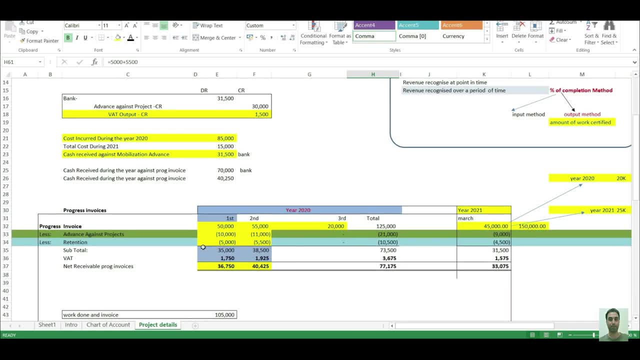 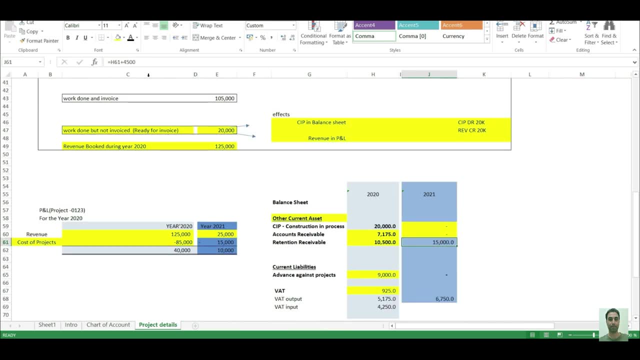 retention receivable. how does it work as far as retention receivable is concerned? you have booked this one, this one, 10,500 and 4,500, so just add your opening balance plus 4,500. so in this year, 2020, your receivable will be shown as 15,000. 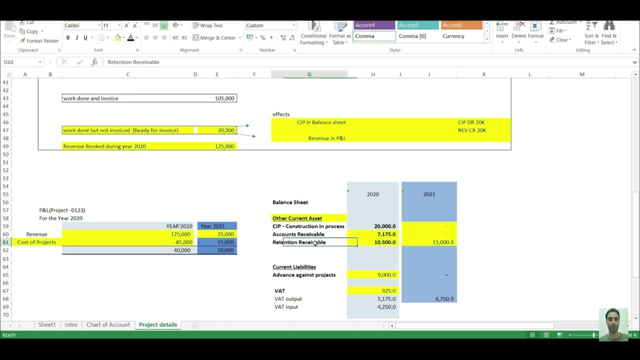 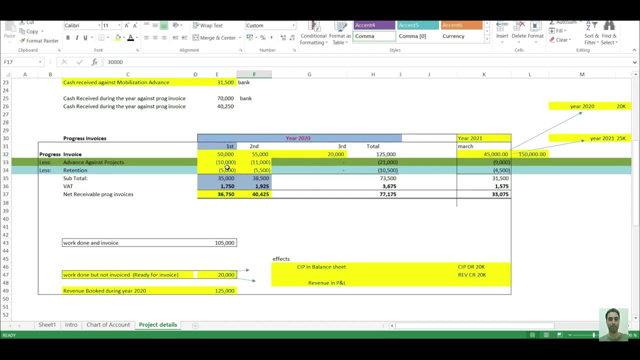 because you haven't invoiced yet, you haven't received yet, so it will be as far your receivable, retention receivable, okay. now, if you see that in the beginning of this project you have booked an advance of 30,000, okay, from this 30,000 you have reduced one by one and with the first invoice you have reduced 10,000 with the. 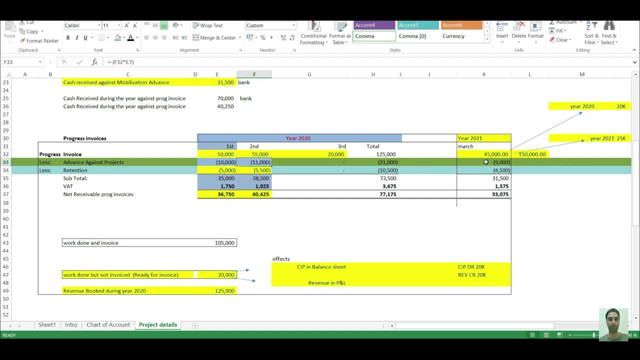 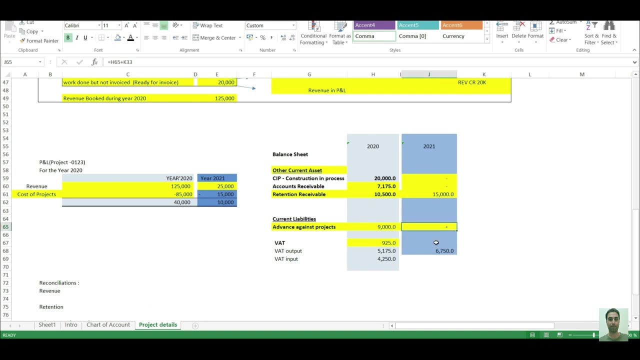 second invoice you have reduced 11,000. with the third invoice you have reduced 9,000. so all this is equal to how much is equal to this plus 30,000? so you have reduced all your, you have consumed all your advance. so it is now zero. now, as far as VAT is concerned, 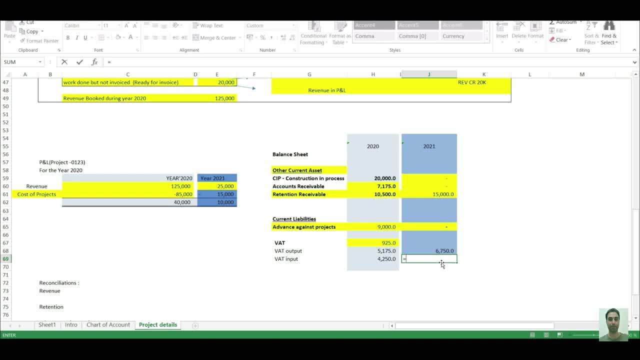 okay, so this month this year you have expenses of 15,000, so 15,000 then to this is your input. okay, minus 0.05. I'm just assuming for the sake of your understanding. okay, so plus. I am assuming that you haven't paid anywhere to the government till yet. okay, so let's see your. 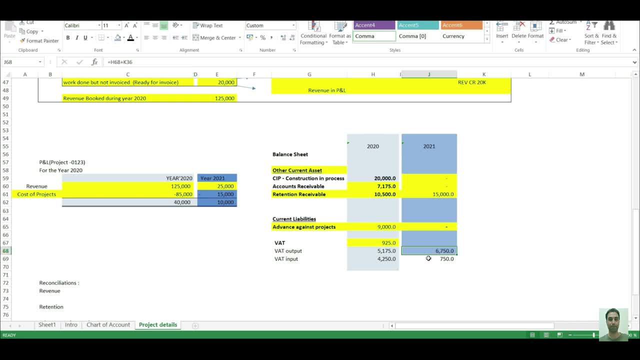 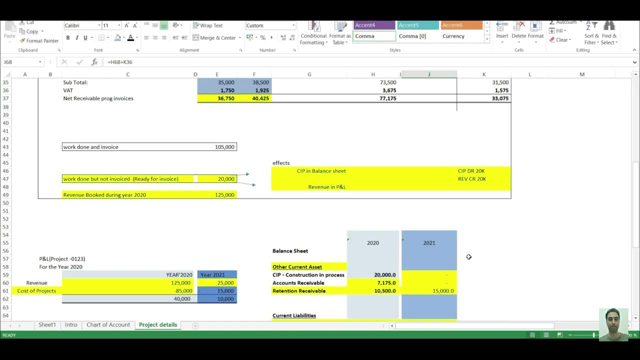 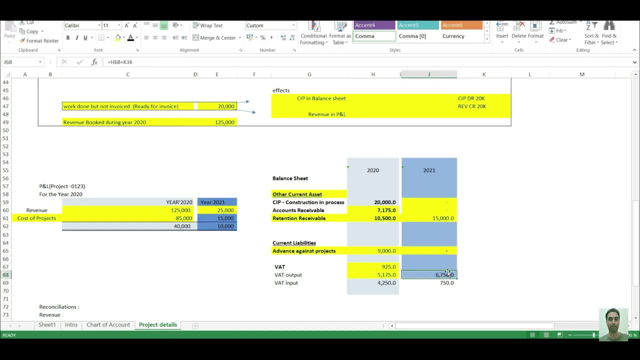 we come up with this. you already know, I have explained to you. now, with this we will add this VAT 1500, 750. so it will become like this: okay, and as far as VAT input is just hypothetical and I have put it, okay, so 6,750 is the VAT output. 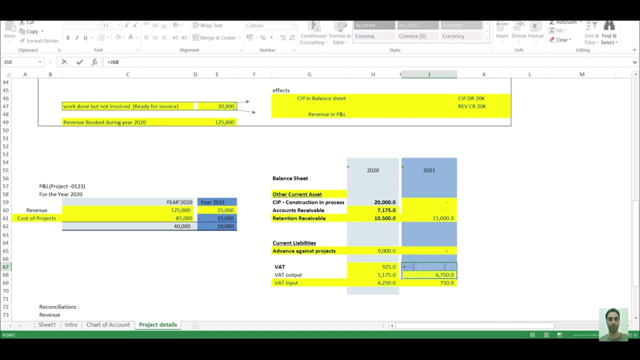 okay, let me add this: plus opening balance. let me add this: okay, now you should concentrate on this VAT output only, okay, not. you should concentrate on this VAT output only, okay, not. you should concentrate on this VAT output only, okay, not VAT net liability, because this is what 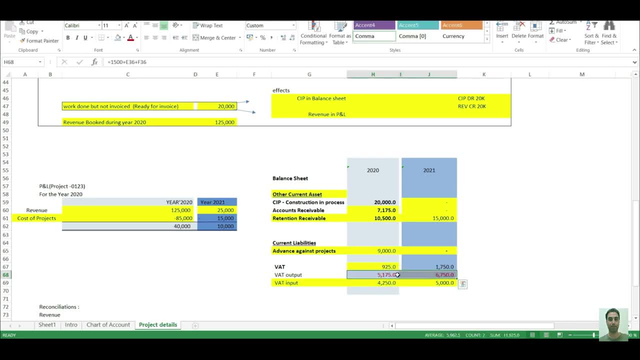 VAT net liability, because this is what VAT net liability? because this is what our concern area is: that this is a net. our concern area is that this is a net. our concern area is that this is a net figure, so don't bother about this, okay figure. so don't bother about this, okay. 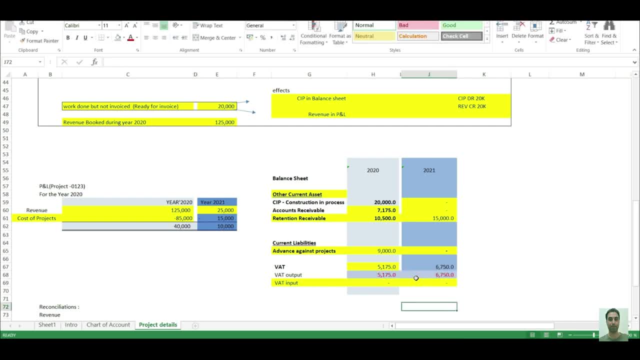 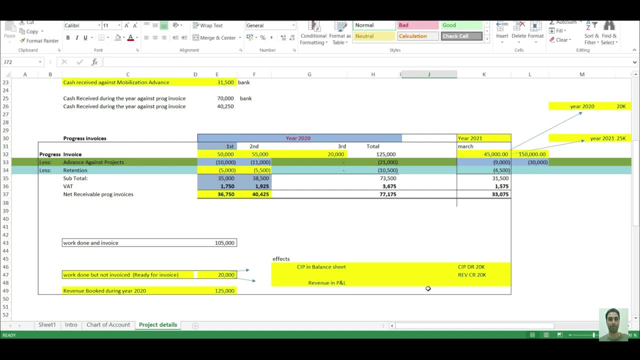 figure, so don't bother about this. okay, let me remove this all together. okay, let me remove this all together. okay, let me remove this all together, okay, okay, all right now, what else? yeah, we have okay, all right now, what else? yeah, we have okay. all right now, what else? yeah, we have performed this everything. yes, yes, so. 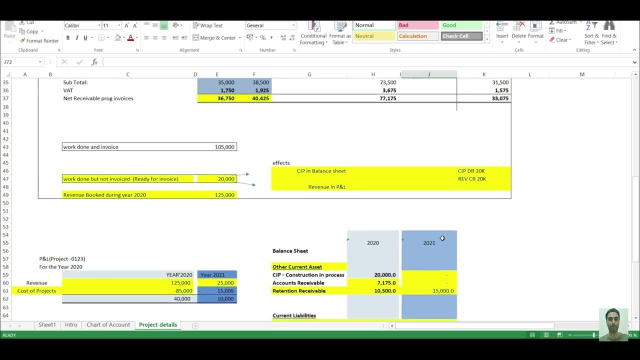 performed this everything, yes, yes. so performed this everything, yes, yes. so now, let's see now, let's see now, let's see what happens. is that that now? let us what happens. is that that now? let us what happens. is that that now? let us reconcile one by one what happens to. 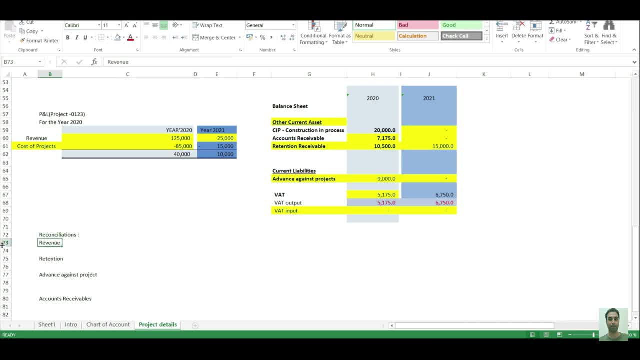 reconcile one by one what happens to reconcile one by one what happens to everything. either we have recorded everything, either we have recorded everything, either we have recorded correctly or not. let's recognize start correctly or not. let's recognize start correctly or not. let's recognize start with the revenue. so this is very 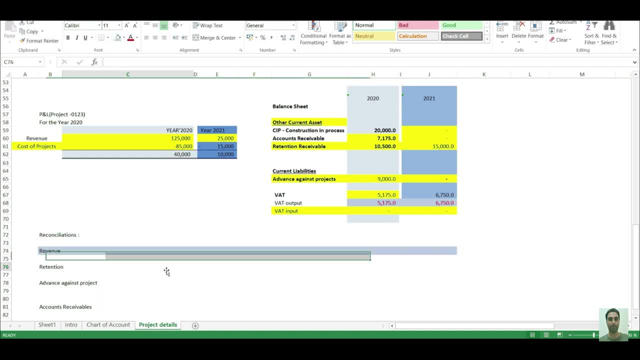 with the revenue. so this is very with the revenue. so this is very important. don't leave, just see how it important. don't leave, just see how it important. don't leave, just see how it works. okay, first of all, let's check our works. okay, first of all, let's check our. 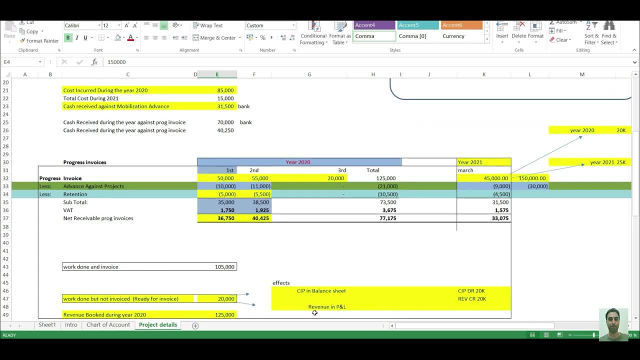 works. okay. first of all, let's check our revenue: total revenue that we are revenue. total revenue that we are revenue. total revenue that we are supposed to record was 150. have we supposed to record was 150. have we supposed to record was 150. have we recorded 150? let's see we have recorded. 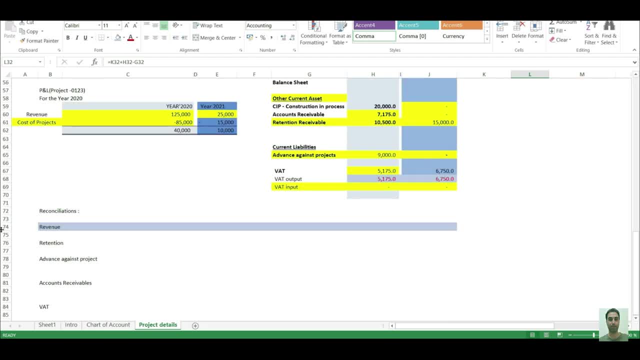 recorded 150. let's see we have recorded recorded 150. let's see we have recorded 150. so it is correct. revenue done any 150, so it is correct. revenue done any 150, so it is correct, revenue done. any question regarding revenue you can ask. 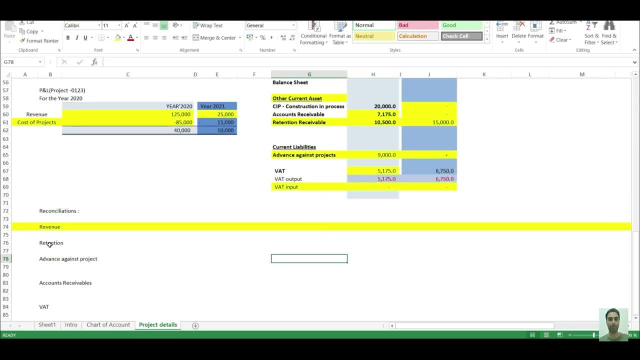 question regarding revenue. you can ask question regarding revenue. you can ask in comment. it is done okay after the in comment. it is done okay after the in comment. it is done okay after the revenue. the next thing is retention revenue. the next thing is retention revenue. the next thing is retention. please bear with me. see over here how we 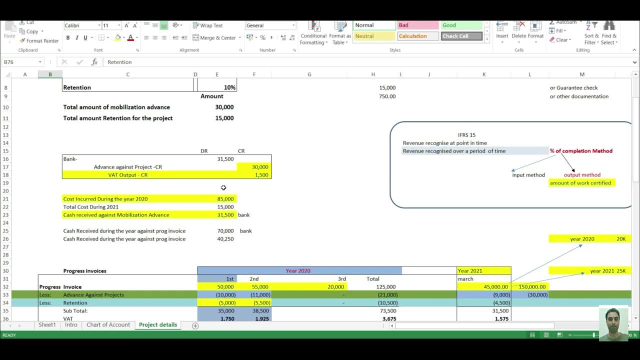 please bear with me see over here how we please bear with me see over here how we will deal with the retention. okay, total will deal with the retention. okay, total will deal with the retention. okay, total retention of the project was how much? retention of the project was how much? 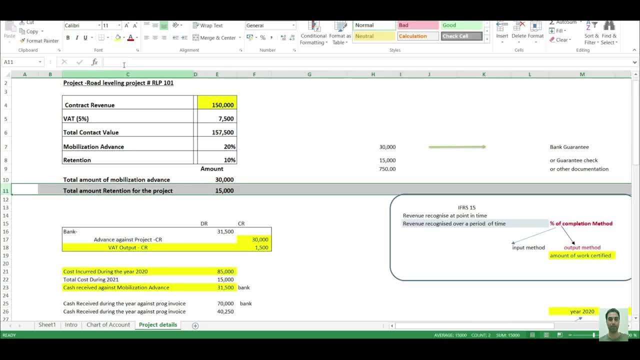 retention of the project was how much? where is this retention amount was 15,000. where is this retention amount was 15,000. where is this retention amount was 15,000. have we booked the retention? what is the? have we booked the retention? what is the? 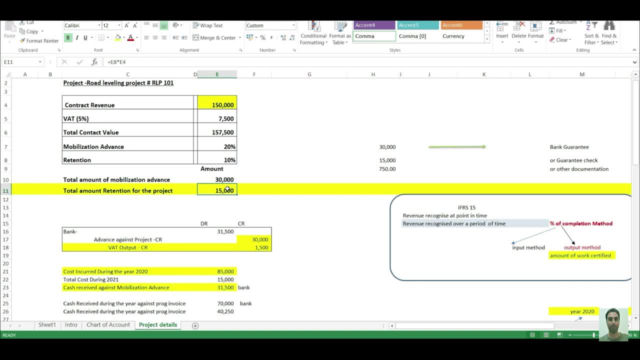 have we booked the retention? what is the status of retention? have we booked 15,000? status of retention. have we booked 15,000? status of retention. have we booked 15,000? have we received 15,000? what is the what? have we received 15,000? what is the what? 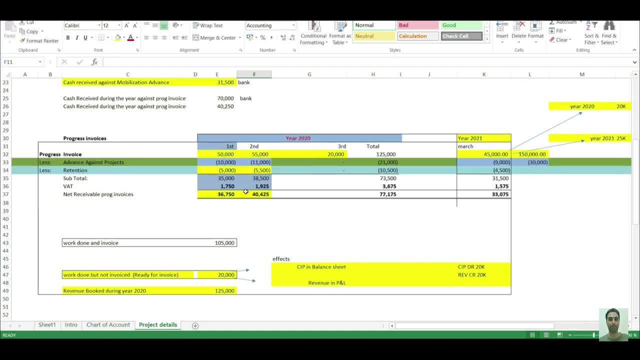 have we received 15,000? what is the? what is this? what about this, let me let us? is this, what about this, let me let us? is this? what about this? let me, let us check it. okay, it should be 15,000 our. check it. okay, it should be 15,000 our. 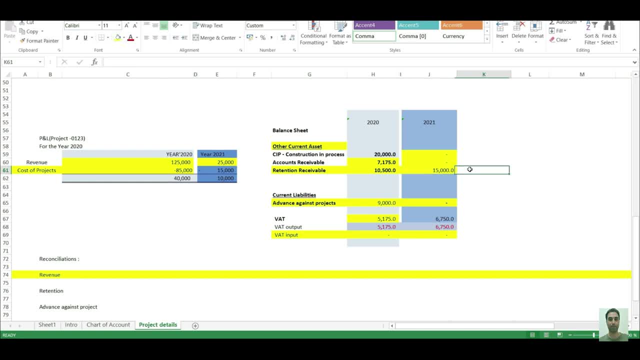 check it. okay, it should be 15,000. our balance sheet shows that 15,000. balance sheet shows that 15,000. balance sheet shows that 15,000 retention. so what will happen once we retention? so what will happen once we retention? so what will happen once we will, once we will invoice for retention? 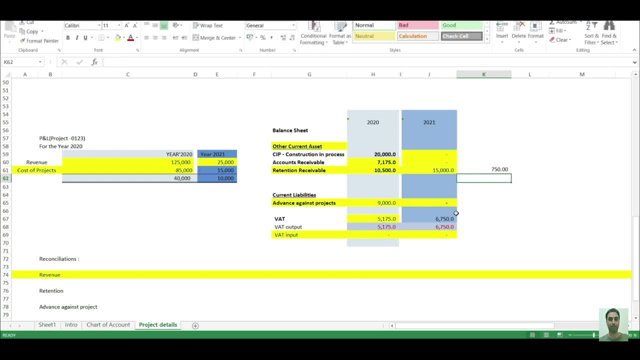 will. once we will invoice for retention will. once we will invoice for retention, we will also charge that, so point zero. we will also charge that, so point zero. we will also charge that, so point zero. file. so that will be 750 at that time file. so that will be 750 at that time. 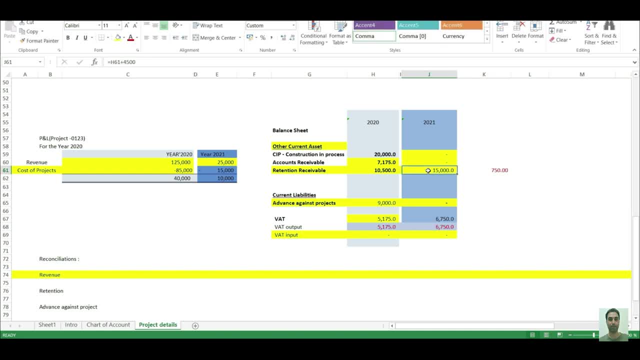 file. so that will be 750 at that time. okay, just keep it in mind, okay, so, okay, just keep it in mind, okay, so, okay, just keep it in mind, okay. so retention is correct. we have correctly. retention is correct. we have correctly. retention is correct. we have correctly charged the retention. okay, total. 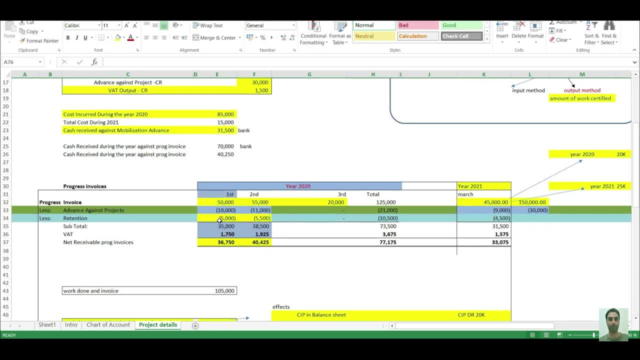 charged the retention. okay, total charged the retention. okay, total retention. you can see over here as well. retention, you can see over here as well. retention, you can see over here as well. okay, let's see here retention: 5, 5, 5, 4, 5. okay, let's see here: retention: 5, 5, 5, 4, 5. 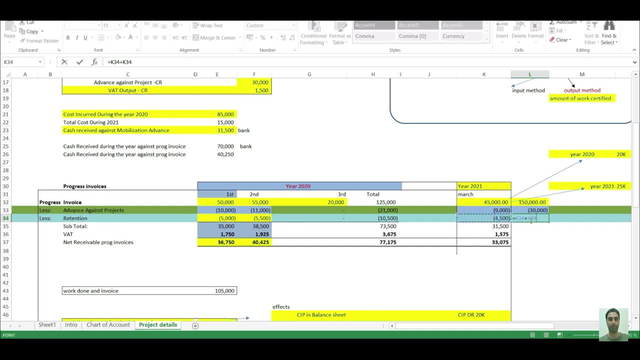 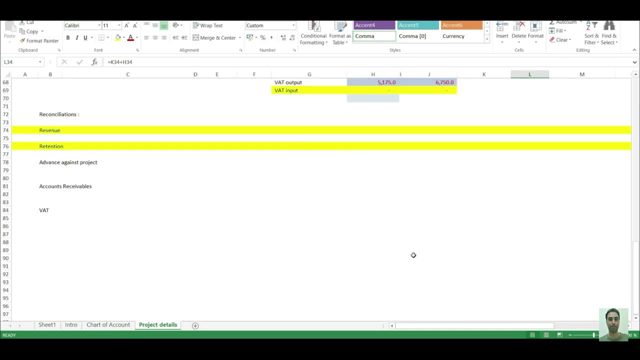 okay, let's see here: retention 5, 5, 5, 4, 5. so is equal to this plus 15,000 we have. so is equal to this plus 15,000 we have. so is equal to this plus 15,000. we have correctly charged. okay, now after. 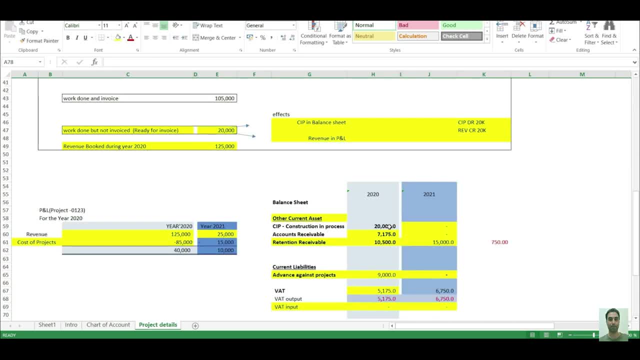 correctly charged. okay now after correctly charged. okay now after. retention advanced against project. let's retention advanced against project. let's retention advanced against project. let's see it once: against: project was 30,000. see it once: against project was 30,000. see it once: against: project was 30,000. without that, with that, 31,500. so let's. 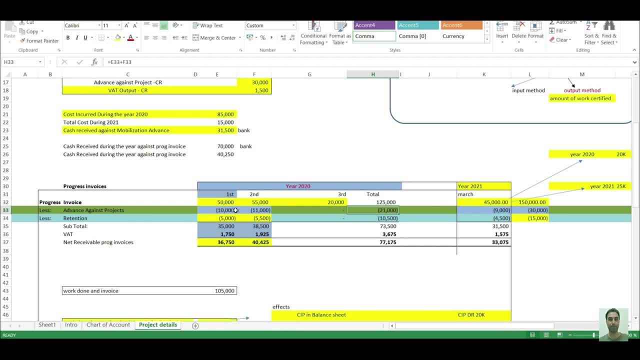 without that, with that 31,500. so let's, without that, with that 31,500. so let's see, we have charged this, this, this. see, we have charged this, this, this. see, we have charged this, this, this, sorry, this, this, this. see, we have charged this, this, this and this, so it is 30,000. we have correct we. 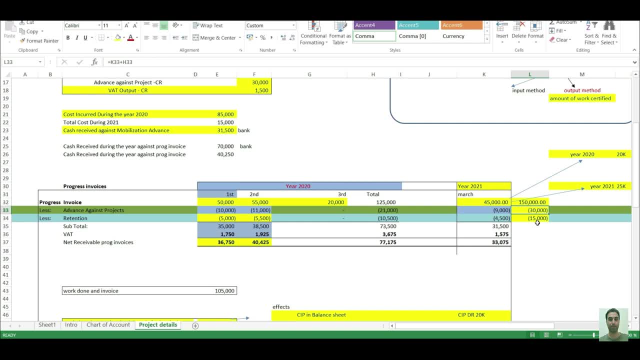 and this, so it is 30,000. we have correct. we and this, so it is 30,000. we have correct. we have correctly charged total total. have correctly charged total total. have correctly charged total total. deducted from them is this and what deducted from them. is this and what. 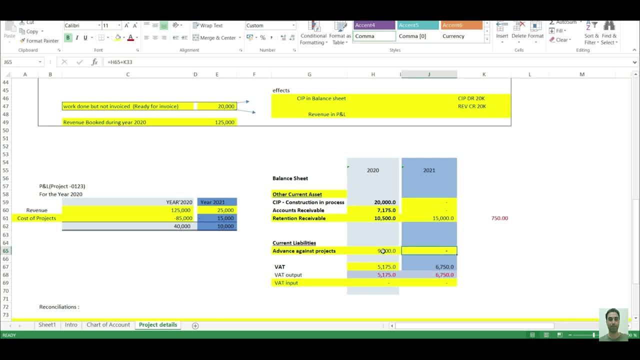 deducted from them is this? and what about the status? it is reduced. we have about the status: it is reduced. we have about the status it is reduced. we have already: 21,000 was reduced in the year of. already 21,000 was reduced in the year of. 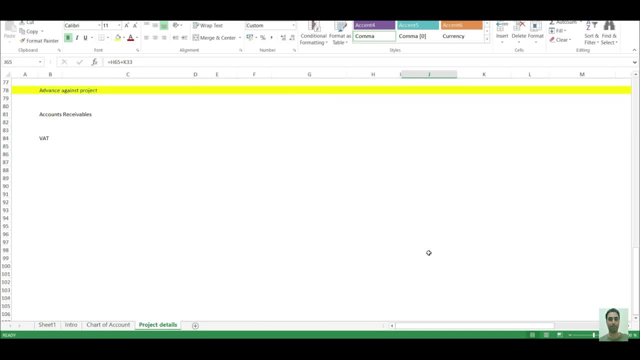 already: 21,000 was reduced in the year of 2020 and 9,000 in the next year. so it is 2020 and 9,000 in the next year. so it is 2020 and 9,000 in the next year. so it is also correct now: account receivable. 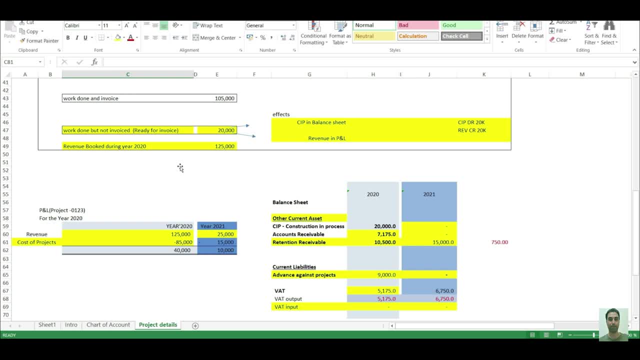 also correct now, account receivable- also correct now, account receivable. let's see account receivable, how it this? let's see account receivable, how it this? let's see account receivable, how it? this is very technical. okay, just look at, that is very technical. okay, just look at that. 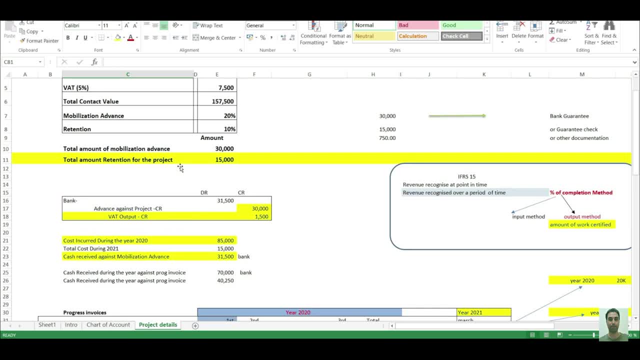 is very technical. okay, just look at that. how does account receivable has worked? how does account receivable has worked? how does account receivable has worked in this scenario? okay, now I will ask you in this scenario. okay, now I will ask you in this scenario. okay, now I will ask you a question. you have performed the work. 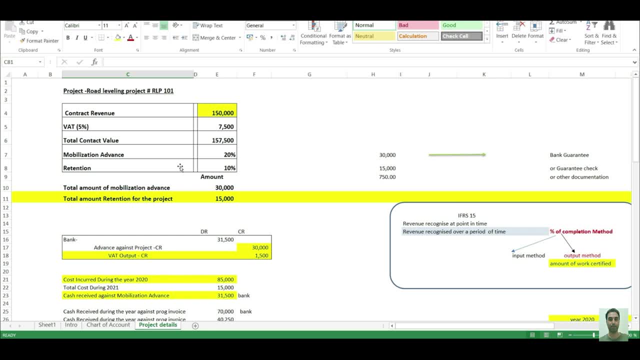 a question. you have performed the work. a question. you have performed the work of 150,000 plus red 7500. you as a manager of 150,000 plus red 7500. you as a manager of 150,000 plus red 7500, you as a manager of my company? I will ask: okay, I'm gonna. 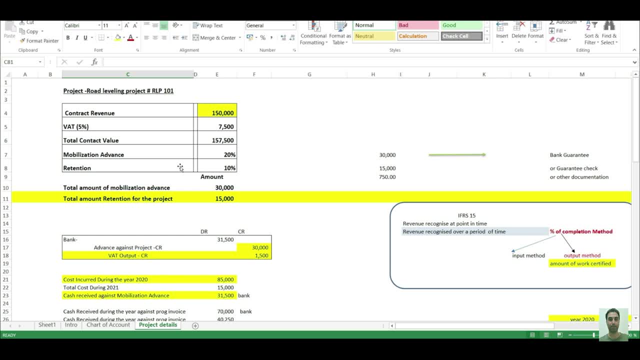 of my company. I will ask: okay, I'm gonna. of my company. I will ask: okay, I'm gonna receive from this customer 157,500. where receive from this customer 157,500? where receive from this customer 157,500? where is that amount? tell me or just explain. 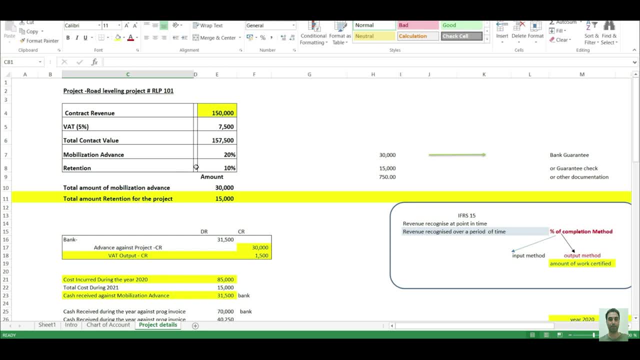 is that amount, tell me or just explain. is that amount, tell me, or just explain it to me? okay, what you will do. I am it to me. okay, what you will do. I am it to me. okay, what you will do, I am gonna show, let's check it. okay, have we? 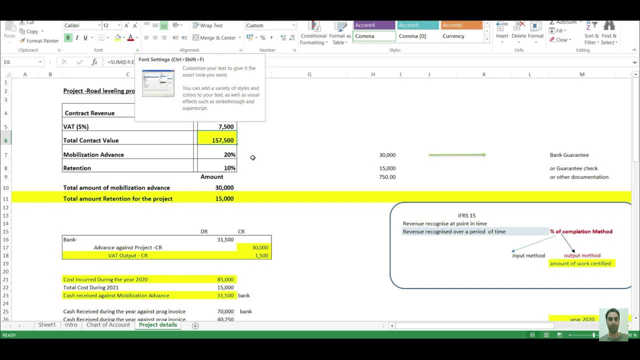 gonna show. let's check it okay. have we gonna show? let's check it okay. have we received or we have booked the received, or we have booked the received or we have booked the receivable for this amount. this is our receivable for this amount. this is our. 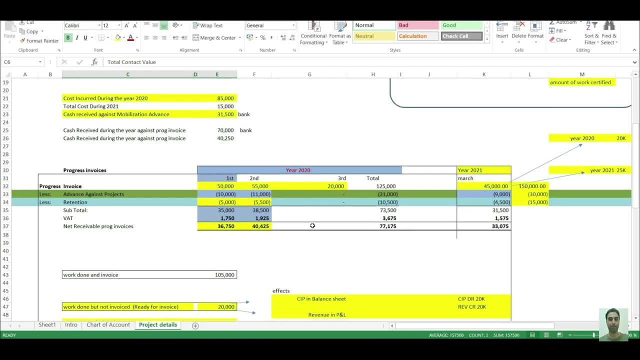 receivable for this amount. this is our concern and when we are dealing with concern, and when we are dealing with concern and when we are dealing with this account receivable thing- okay, let's this account receivable thing. okay, let's this account receivable thing- okay, let's see one by one. so we are looking up for. 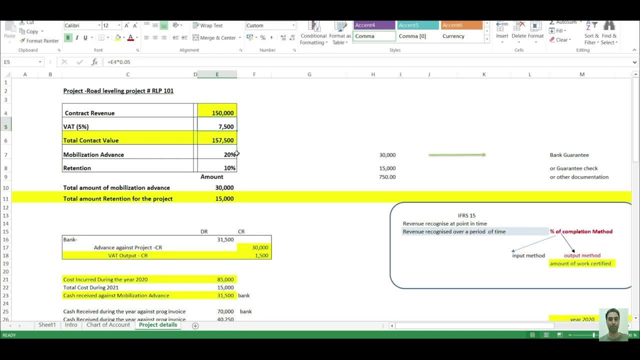 see one by one. so we are looking up for see one by one. so we are looking up for: this value, this value is with that, okay. this value, this value is with that, okay. this value, this value is with that, okay. so keep in mind so total receivable that. 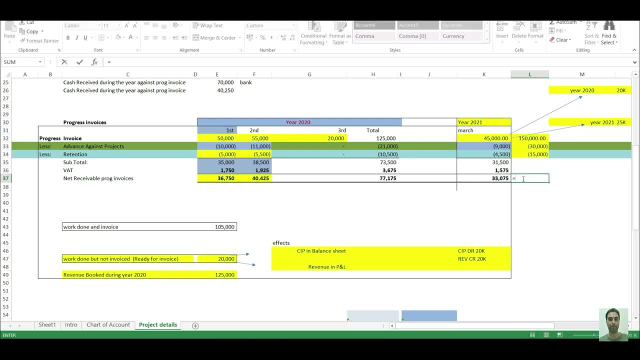 so keep in mind so total receivable that. so keep in mind so total receivable that we booked with an progressive invoice. is we booked with an progressive invoice? is we booked with an progressive invoice? is this plus this, how much with with that? this plus this, how much with with that? 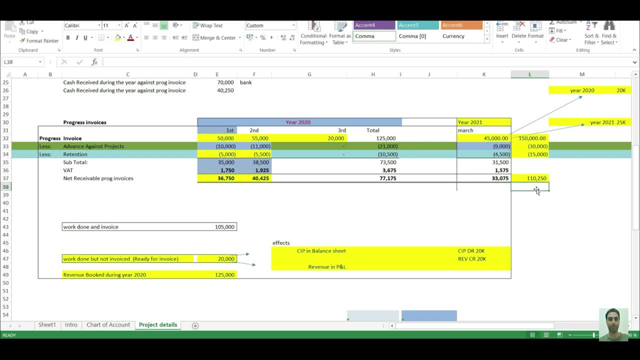 this plus this: how much with with that? how much 110,000 250, right? you will ask. how much 110,000 250, right? you will ask. how much 110,000 250, right? you will ask or no, you or no. you or no, you will ask, or no, you will. 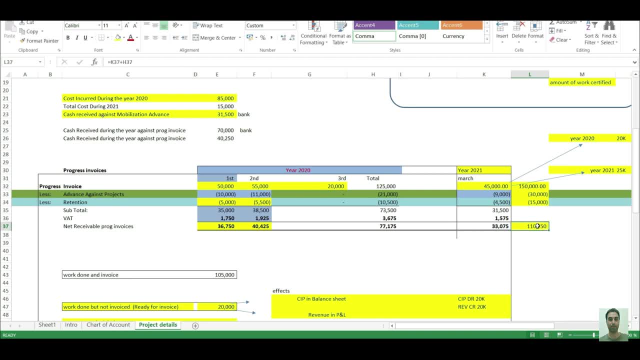 or no. you will ask or no. you will brief your superior that 110,000 250. we brief your superior that 110,000 250. we brief your superior that 110,000 250. we have been asking them to pay us, or you? 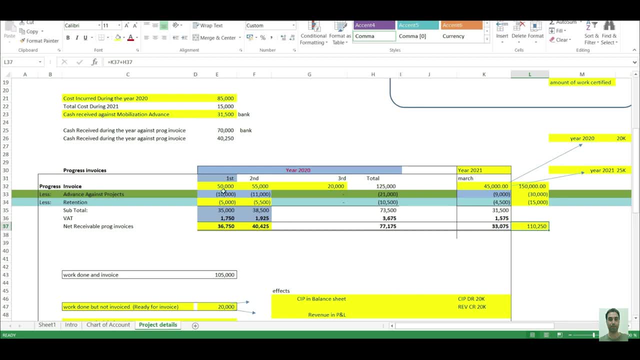 have been asking them to pay us, or you have been asking them to pay us, or you. we have been booking them to pay us one. we have been booking them to pay us one. we have been booking them to pay us one. where it is that you will show him first. 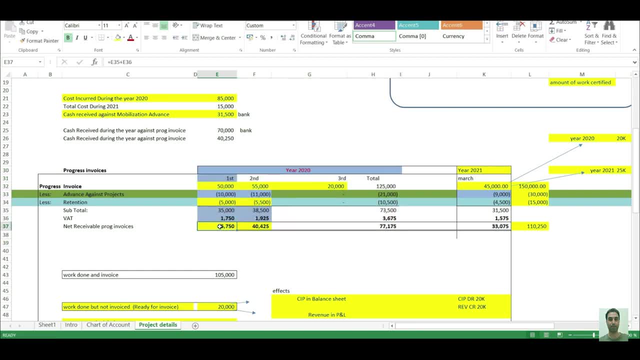 where it is that you will show him first, where it is that you will show him first progressive advice. this one, second, this progressive advice. this one, second, this progressive advice, this one, second, this one. this is what we are asking. give us one. this is what we are asking, give us. 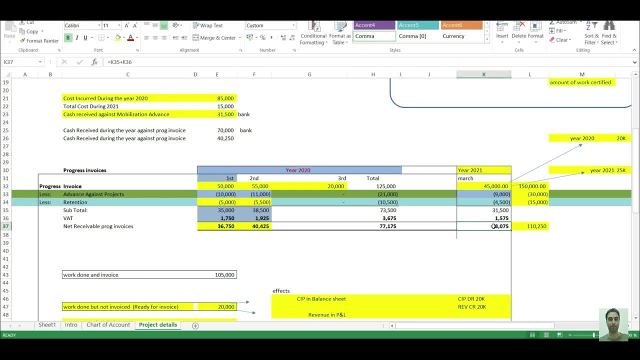 one. this is what we are asking. give us this amount. this is what we are asking. this amount, this is what we are asking. this amount, this is what we are asking: give us this amount. then we are asking: give us this amount. then we are asking: give us this amount. then we are asking: give us this amount. he will say: okay. 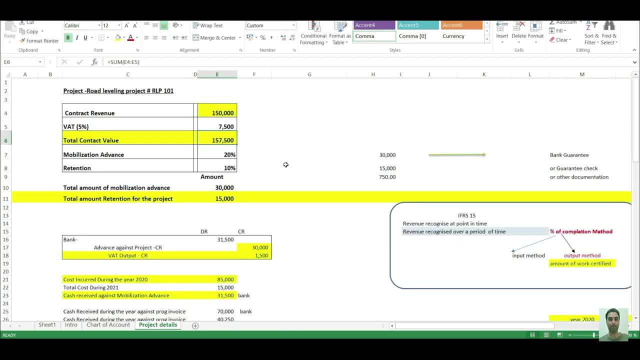 give us this amount. he will say: okay, give us this amount. he will say, okay, this is 110 250. I am supposed to receive. this is 110 250. I am supposed to receive. this is 110 250. I am supposed to receive one: 57 500, including that. you will say: 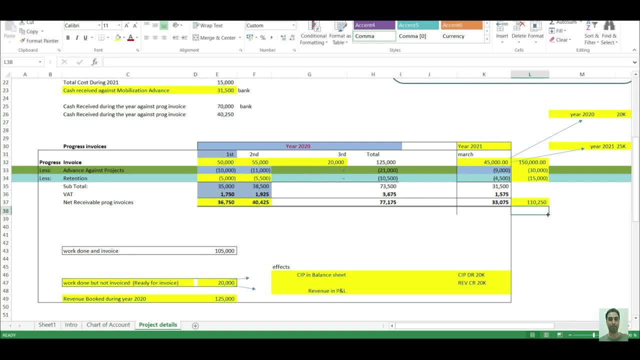 one 57 500, including that. you will say one 57 500, including that. you will say: hold on, then we will invoice them. hold on, then we will invoice them. hold on, then we will invoice them. retention: how much? 15,000, okay, plus wet. 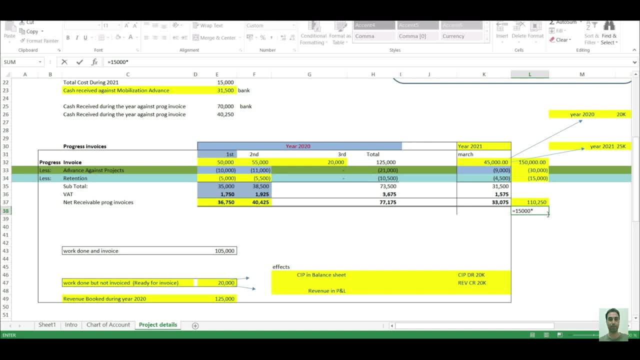 retention: how much 15,000 okay, plus wet. retention: how much 15,000 okay, plus wet. when we will charge 15,000 into. so I am when we will charge 15,000 into, so I am when we will charge 15,000 into. so I am adding at the moment, okay, man to 1.05. so 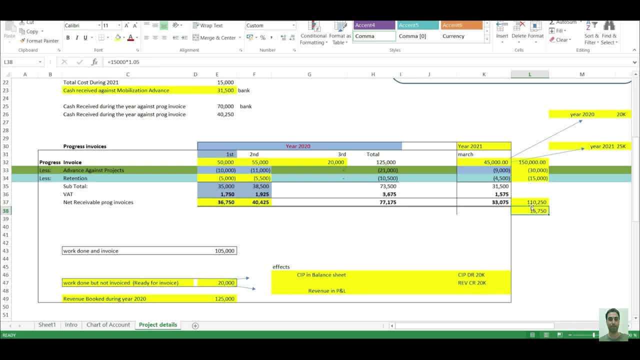 adding at the moment, okay, man to 1.05. so adding at the moment, okay, man to 1.05. so 15,000, 750, we will. you will tell them: we 15,000, 750, we will. you will tell them we 15,000, 750, we will. you will tell them, we will tell your manager that we have all. 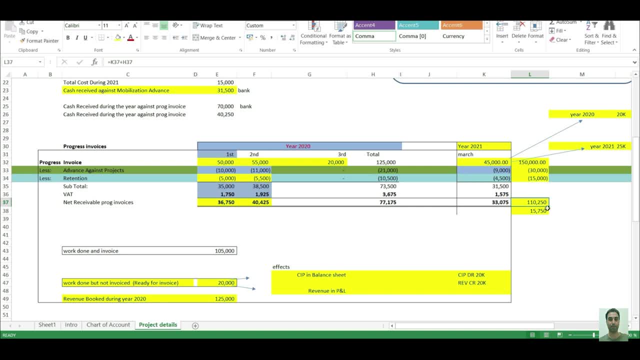 will tell your manager that we have all, will tell your manager that we have all. your boss, who is who doesn't have this? your boss, who is who doesn't have this? your boss, who is who doesn't have this much accounting background? okay, this much accounting background. okay, this. 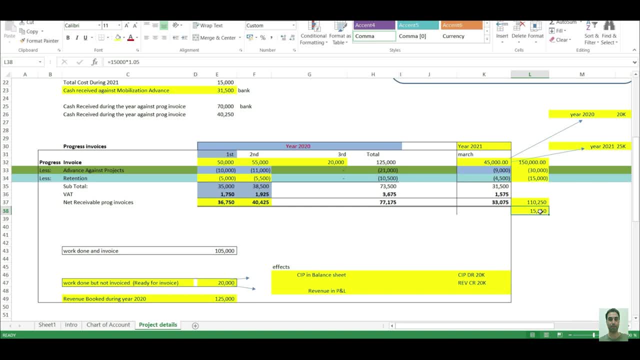 much accounting background. okay, this much. we have already asked them an much. we have already asked them an much. we have already asked them an element term plus. we will ask them this element term plus. we will ask them this element term plus. we will ask them this much. so, how much is this? he will ask you. 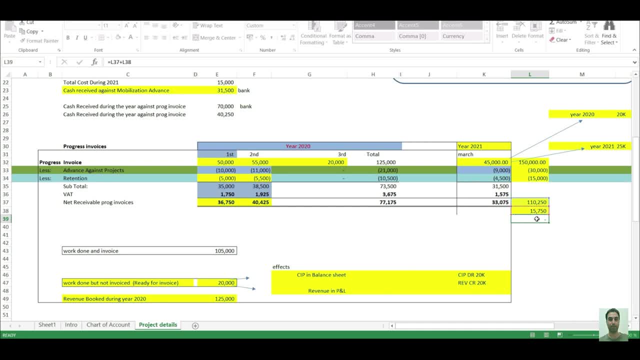 much so how much is this? he will ask you: much so how much is this? he will ask you: okay, how much is this total plus you? okay, how much is this total plus you? okay, how much is this total plus? you will say: this is 126,000. okay, so what? 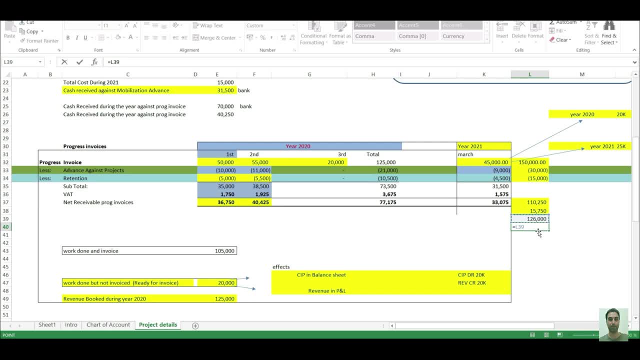 will say: this is 126,000, okay. so what will say? this is 126,000, okay. so what about the remaining amount? you will say about the remaining amount. you will say about the remaining amount, you will say: okay, this 126,000 minus how much is the? 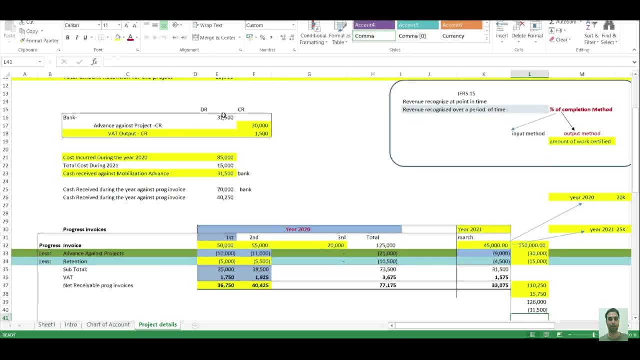 okay, this 126,000 minus. how much is the okay this 126,000 minus. how much is the total amount of the project 157,500. total amount of the project 157,500. total amount of the project 157,500. enter this is 31,500, you will say, sir, we. 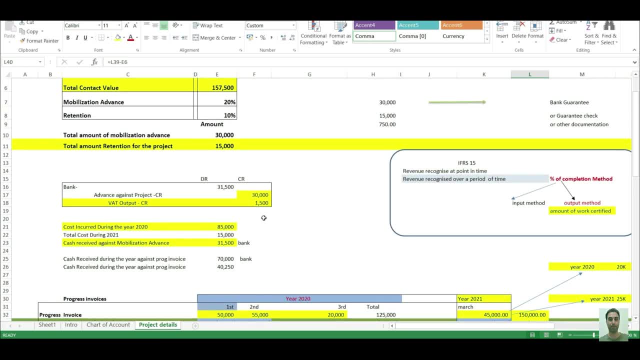 enter: this is 31,500. you will say: sir, we enter this is 31,500. you will say: sir, we have already received this 31,000. in have already received this 31,000. in have already received this 31,000 in advance. 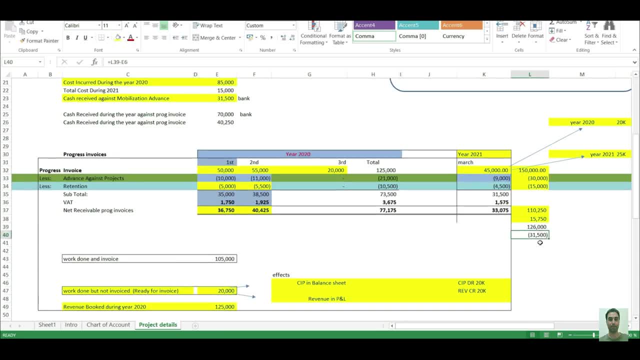 advance, advance. yes, including vitamin. okay, so 31,500. yes, including vitamin. okay, so 31,500. yes, including vitamin. okay, so 31,500. so how much is total now? this sorry is so how much is total now, this sorry is so. how much is total now, this sorry is equal to this plus this, plus this, so 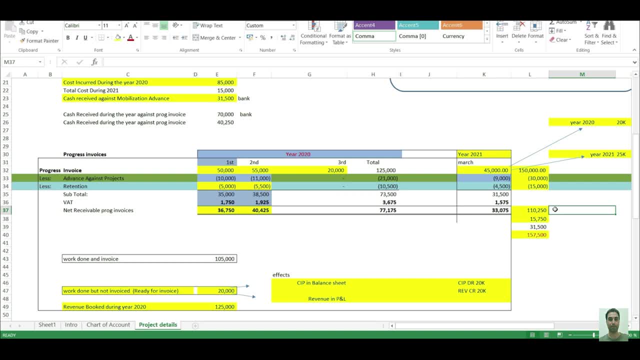 equal to this plus this plus this. so equal to this plus this plus this. so 157,000 is your tallied amount. what is 157,000 is your tallied amount? what is 157,000 is your tallied amount? what is this? this is progress. seven, wise, you can. 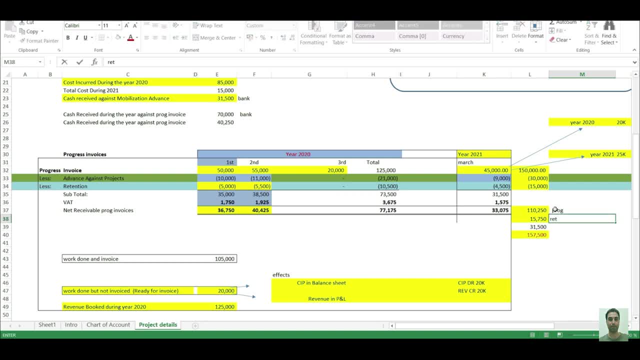 this. this is progress, seven wise. you can this. this is progress, seven wise. you can say to him this is say to him this is say to him: this is the retention we will receive after six, the retention we will receive after six, the retention we will receive after six month. okay, this is what this is. this was. 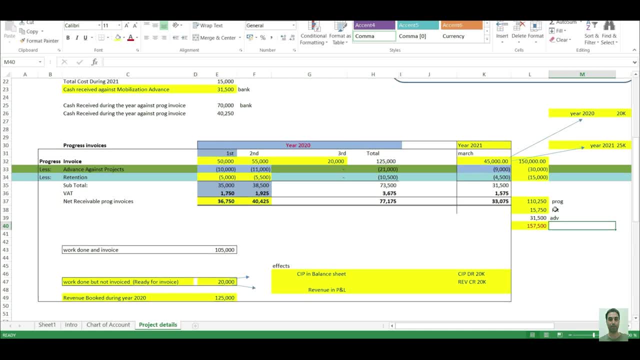 month: okay, this is what this is. this was month. okay, this is what this is. this was that. once we receive. so, sir, we are that. once we receive. so, sir, we are that. once we receive. so sir, we are correct. okay, now, your advance is also correct. okay, now your advance is also. 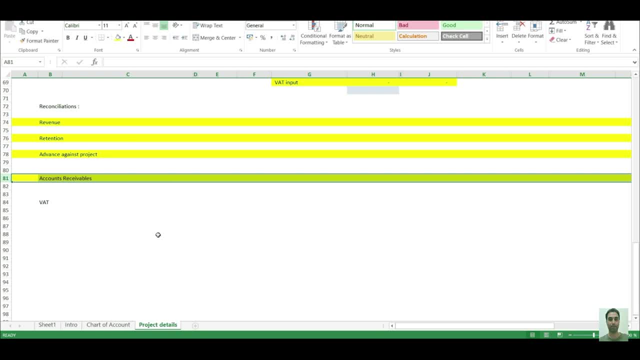 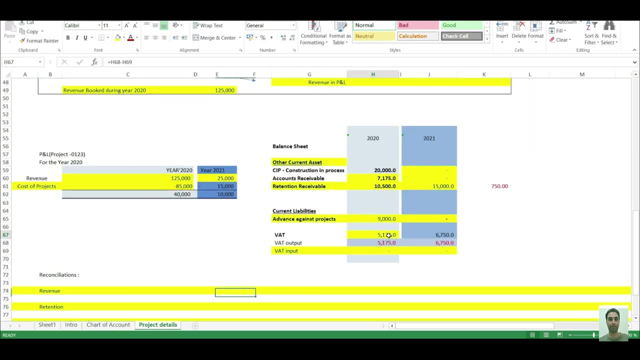 correct. okay, now your advance is also. counter civil is also valid, or counter civil is also valid, or counter civil is also valid, or reconcile now going for the fact. all reconcile now going for the fact. all reconcile now going for the fact. all right, all right now as far as that is. right. all right now. as far as that is right, all right now. as far as that is concerned. I have already explained to you concerned. I have already explained to you concerned, I have already explained to you, but I will explain once one more time. but I will explain once one more time. 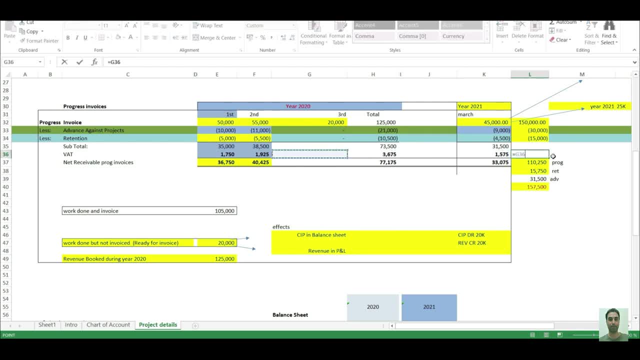 but I will explain once one more time. this is a total VAT that we have charged. this is a total VAT that we have charged. this is a total VAT that we have charged them with the progressive invoice, this them with the progressive invoice, this them with the progressive invoice. this, sorry, is equal to this plus this: how? 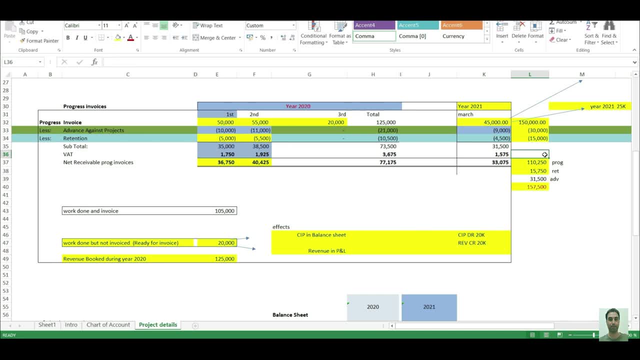 sorry is equal to this plus this. how sorry is equal to this plus this. how much five to five zero. this is the VAT much five to five zero. this is the VAT much five to five zero. this is the VAT with progressive invoice: okay, plus with. with progressive invoice: okay, plus with. 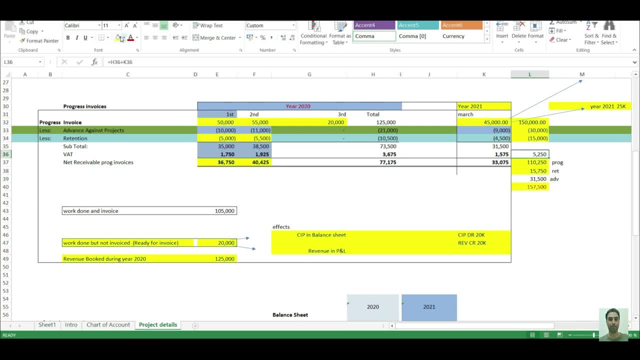 with progressive invoice. okay, plus with that once, how much you have charged this, that once, how much you have charged this, that once, how much you have charged? this is with the progressive invoice but and is with the progressive invoice but and is with the progressive invoice but. and what about at once, how much it is where? 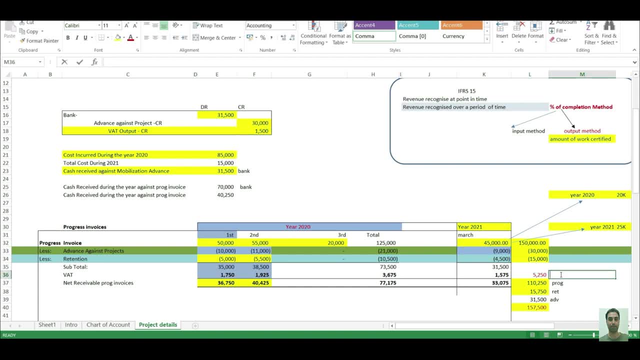 what about at once, how much it is where? what about at once, how much it is where it is? yeah here, 1500, 1500. okay with this. it is yeah here, 1500, 1500. okay with this. it is yeah here, 1500, 1500. okay with this is with progressive invoice. this is with. 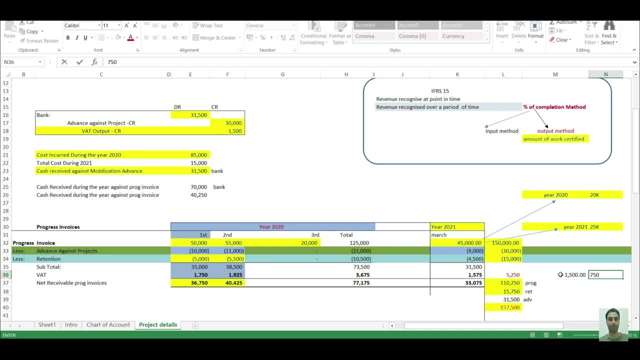 is with progressive invoice, this is with is with progressive invoice, this is with advanced. and what about retention 750 advanced? and what about retention 750 advanced? and what about retention 750? okay, so how much is the total? now is okay. so how much is the total now is? 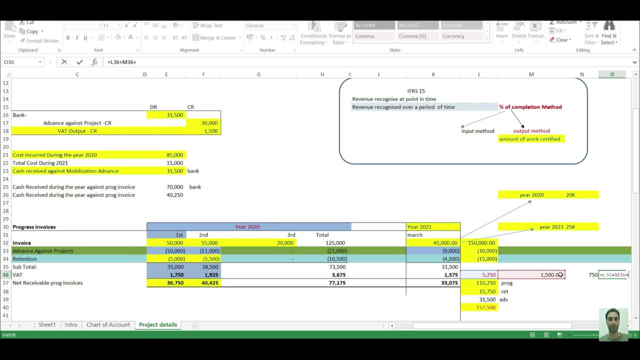 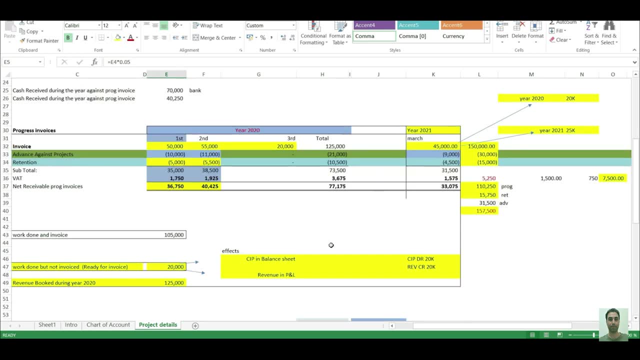 okay, so how much is the total now is equal to this plus this plus this? so how equal to this plus this? so how equal to this plus this. so how much is 7500 and how much it is here. so this is much is 7500 and how much it is here. so this is. 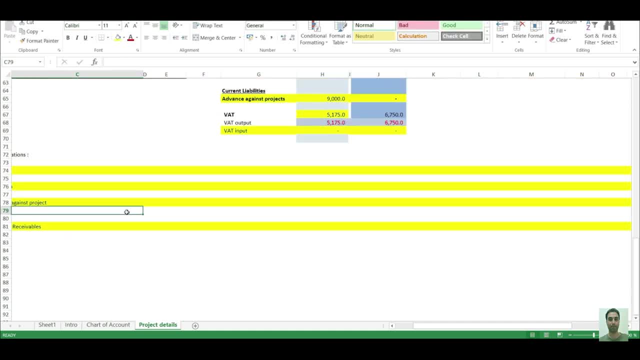 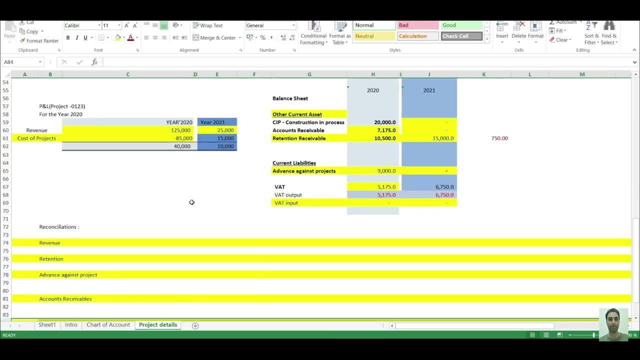 much is 7500 and how much it is here. so this is how: how much is 7500 and how much it is here. so this is how it worked. so our vat is it worked. so our vat is it worked. so our vat is. also tell it inside: okay, so that is it. that's how it. 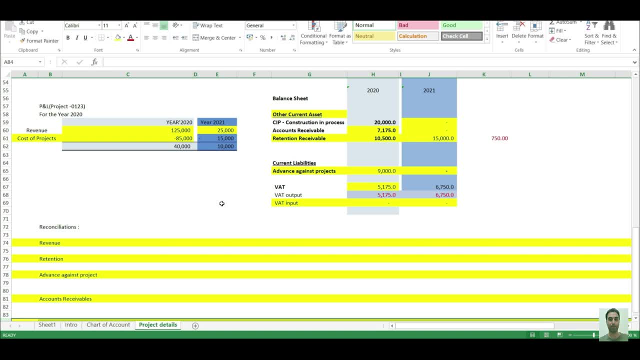 also tell it inside, okay, so that is it. that's how it also tell it inside, okay, so that is it. that's how it was. so I hope you understand this was so. I hope you understand this was so. I hope you understand this video and it helped you. please click the. 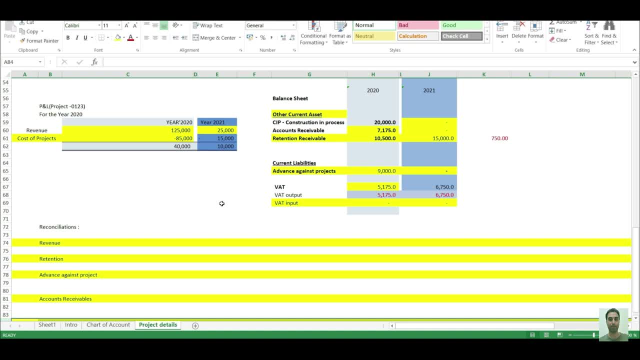 video and it helped you. please click the video and it helped you. please click the subscribe button from share with your subscribe button. from share with your subscribe button. from share with your friends. like this video and give me friends like this video. and give me friends like this video and give me thumbs up so I can release this side of. 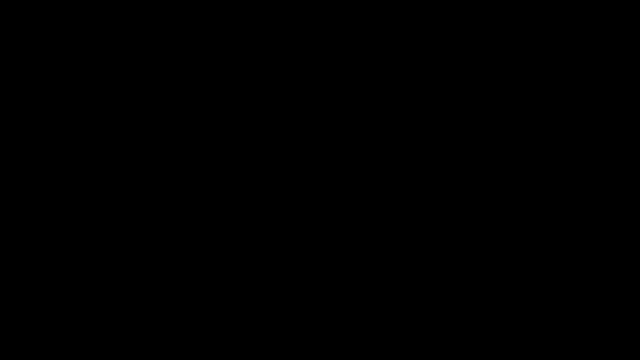 thumbs up so I can release this side of thumbs up, so I can release this side of more videos. thank you very much. take more videos. thank you very much. take more videos. thank you very much. take care. 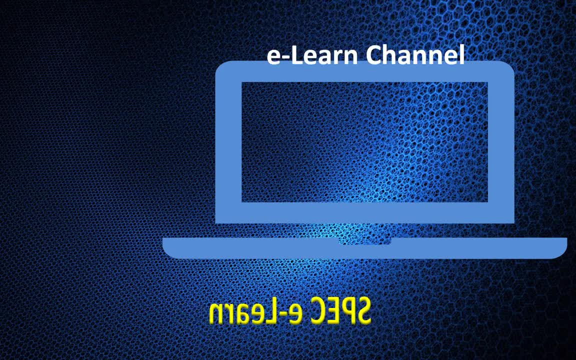 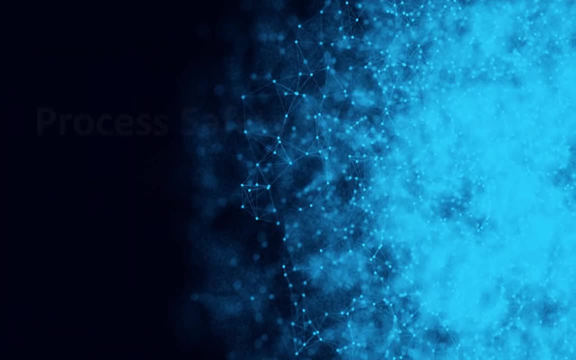 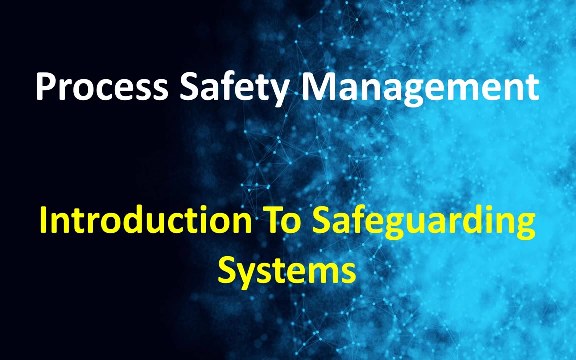 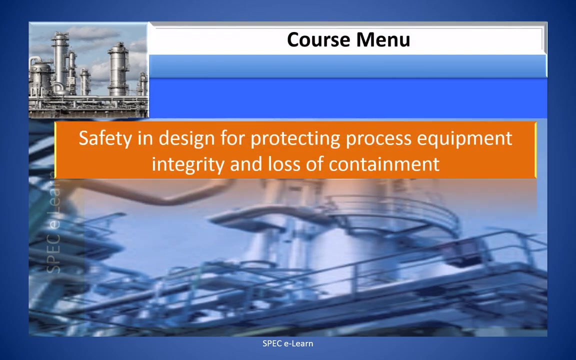 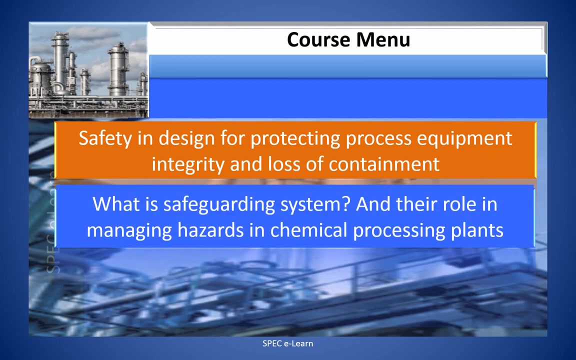 Hello everyone, welcome to SPECT eLearn, the online learning channel dedicated to chemical engineers. In this video course, you will learn safety and design for protecting process equipment, integrity and loss of containment. What is safeguarding system and their role in managing hazards in chemical processing plants.